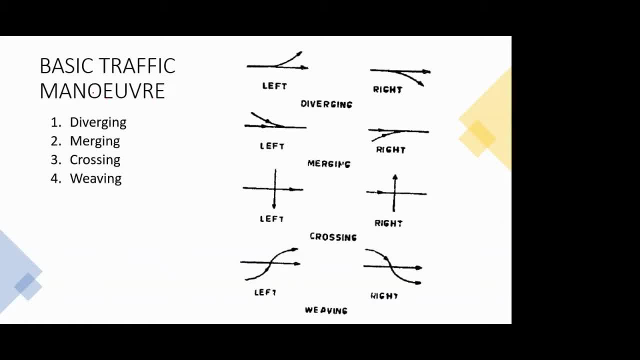 So till now what we have seen is the parameters of traffic, then its interrelationship, then we had seen the traffic studies in detail. So now we know that traffic is. Traffic is nothing but movement of your vehicles or pedestrians on road. 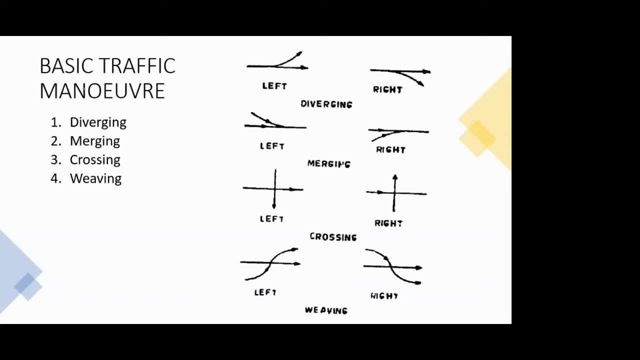 So if we concentrate only on the movement of vehicles, so we can come up with basic traffic maneuvers, what are shown here, the four basic traffic maneuvers, that is, diverging maneuver, Traffic maneuvers are nothing. but if I assume that two vehicles are traveling from two different directions, so how will they? 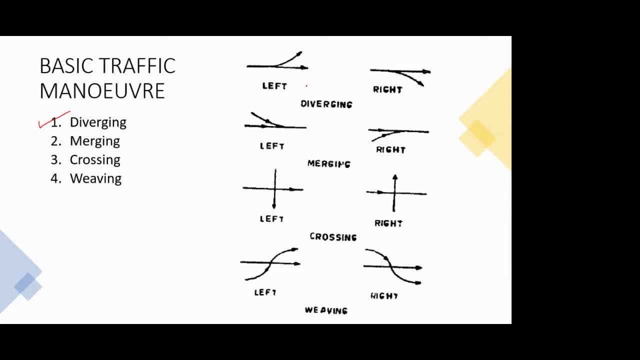 cross each other or what will be the interaction between them, So that you can say as a traffic maneuver or not if two vehicles, even if a single vehicle, then two- how it moves on the road, So that is covered in this traffic maneuver. 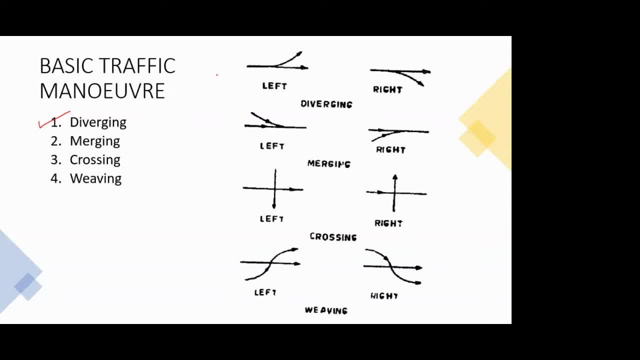 So first is the diverging one. diverging maneuver: So you can see the top figure on the right side. So both the types of maneuvers are shown, the left and the right. So diverging it is nothing, but you are not actually taking a turn. 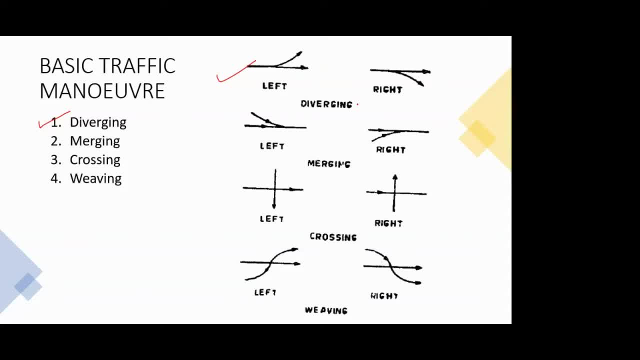 It is not complete 90-degree turn or U-turn, but it is just a sort of branching kind of thing. So that is the diverging maneuver. Then, similarly, you have a merging maneuver. Now diverging and merging you will predominantly see in highways or expressways, where you have controlled access. controlled access as in 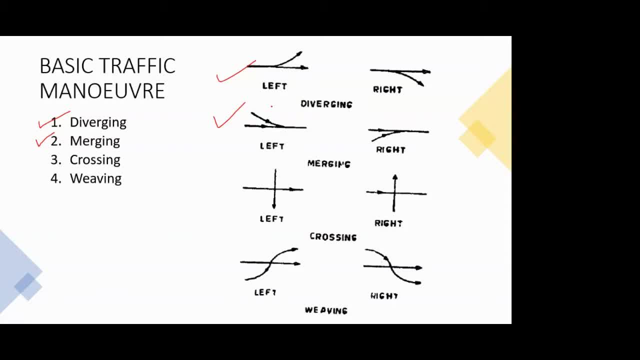 Anyone cannot enter the highway. Anyone cannot enter the highway or the expressway at any location he or she desires, But there are specific locations only at which you can enter the highway. So the best example now: most of you have traveled in and around Pune. 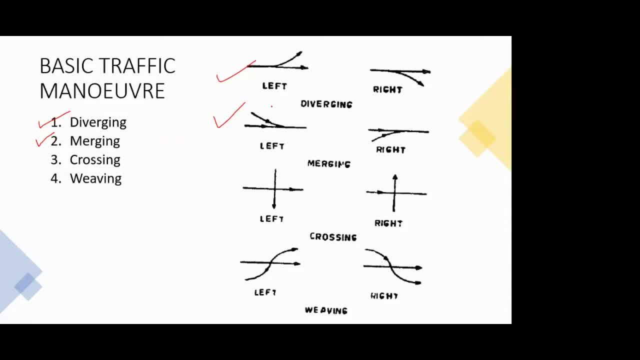 So, assuming that you have traveled on Mumbai-Pune expressway, So that is a controlled Access, controlled expressway, as in- only at specific locations you can enter the expressway and only at specific locations you can exit. So, on that exit and entry, whatever is the maneuver of your vehicle that is diverging and merging. 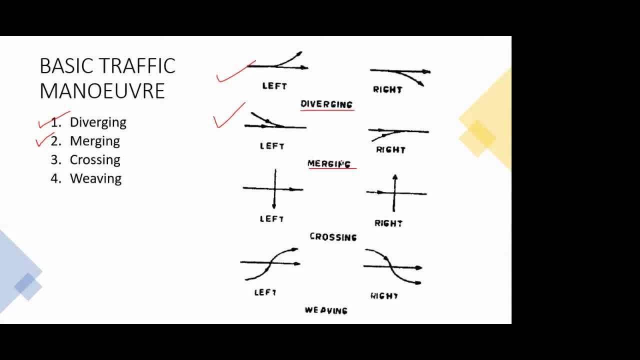 So merging is whenever you are entering that access controlled expressway, that is merging, And whenever you are leaving it. so that is a diverging maneuver. Crossing maneuver you will predominantly see in add-grade intersections, So we will come to that later. what is an add-grade intersection? 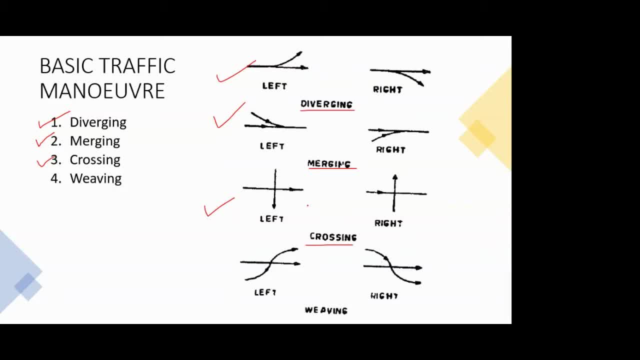 But for now just remember that Crossing maneuver. mainly it comes into picture when you have an add-grade intersection And then two vehicles traveling in two different directions. they are supposed to cross each other's path, So that is a crossing maneuver. 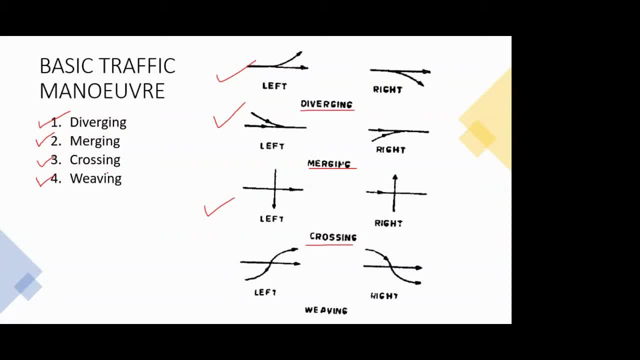 And then there is a slight advancement over the crossing maneuver. That is the fourth one, that is weaving maneuver. This also we will see in next couple of slides when we see the rotary intersection. So there is a difference between crossing and weaving. 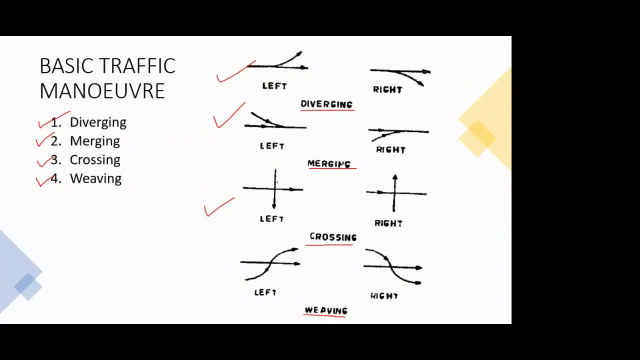 As in, crossing is nothing, but as you can see here in the picture, They cross- not maybe at a perpendicular, or we will assume that almost it is crossing at a perpendicular And one of the vehicle has to stop in order for the another vehicle to cross. 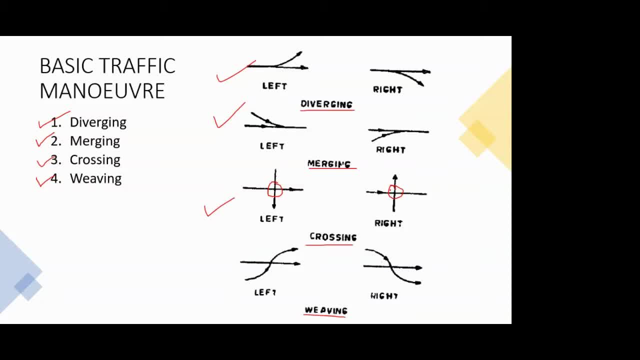 We will assume that or not even stop. So at least the driver has to reduce the speed significantly so that the other vehicle passes In weaving maneuver. what happens is it is sort of a crossing maneuver Because you can see the paths are again crossing over here. 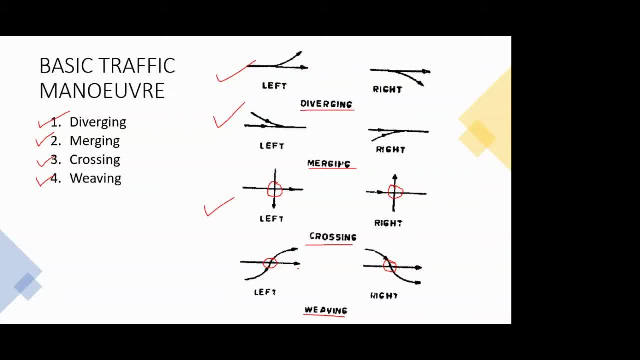 But now, in this case, instead of one vehicle stopping and the other moving, Or one vehicle slowing down and the other going fast, What is done in weaving is the width of the road is controlled in such a way, And the radius is controlled in such a way, that 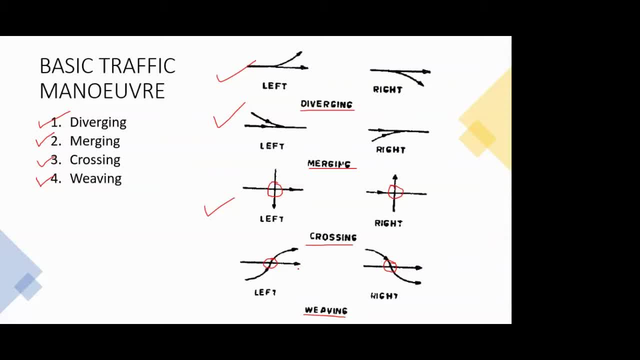 both the vehicles, they will reduce their speed a bit, Or we are controlling as a designer, we are controlling their speeds And then both the vehicles can move simultaneously and cross each other's path. So that is the weaving maneuver. So this we will see from example, when you, when I, discuss the rotary intersection. 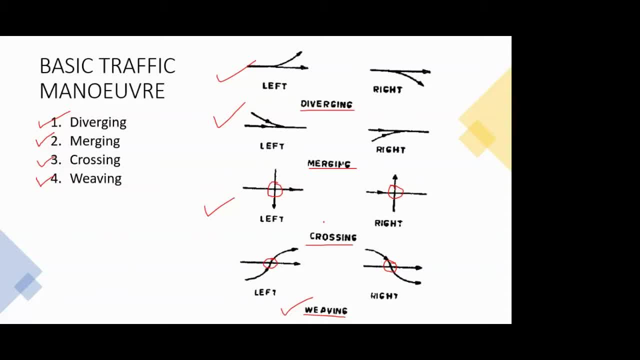 So these are the four basic maneuvers And for understanding the working of the vehicle, Of any interchange or any intersection, You need to understand what will be the movement of the vehicles over there. So that is why I have shown this slide. 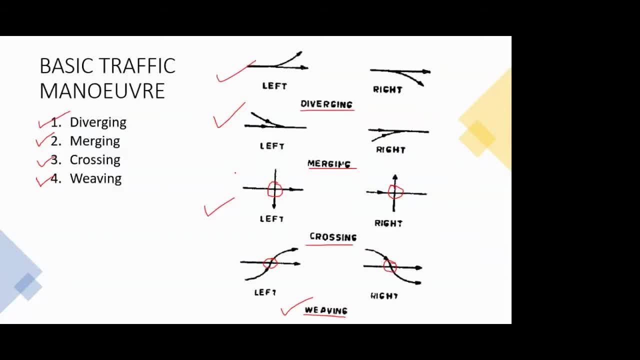 And something related to maneuvers. So, as I told you, in crossing, if you concentrate on this, So whenever two vehicles are going to cross each other at this 90 degree, Or maybe at some angle, So this is termed as a conflict point. 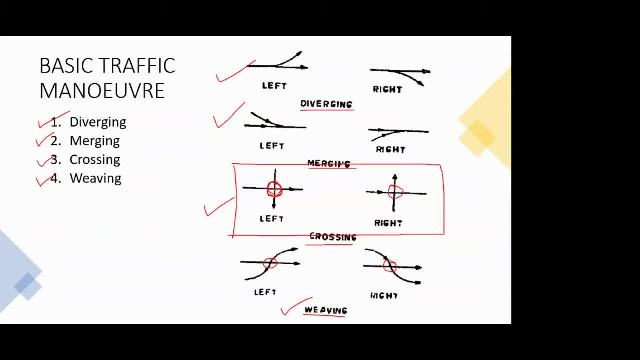 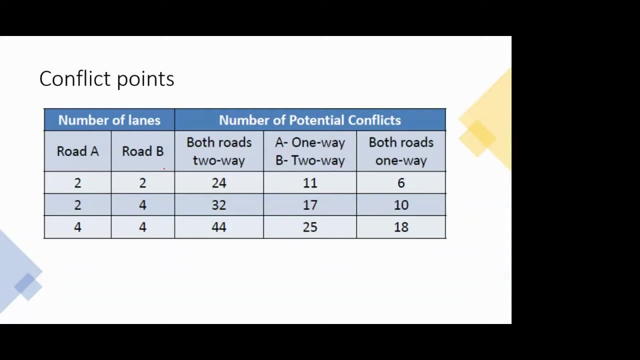 Conflict point, as in: that is the point where there is a chance That if neither of the vehicles slows down, So they are bound to go into an accident. So that is a conflict point. So like that, you can, Not you can, you have to calculate conflict points for a given intersection. 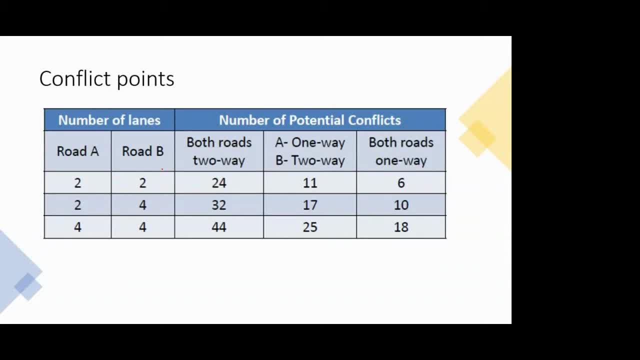 Ad-grade intersection And then if it exceeds, Not exceeds, So if it is having more conflicts, So it is better to reduce those conflicts, As in, if you see this example, Or in this table, I have given an example- that you have two roads. 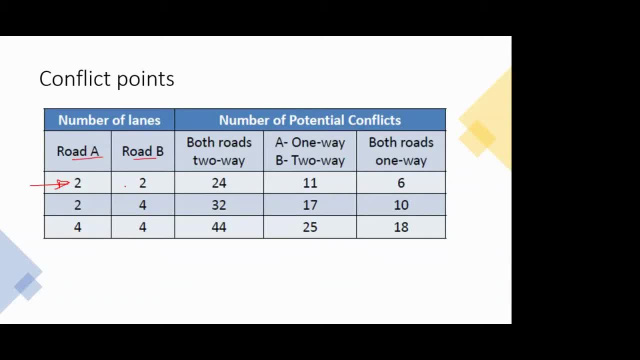 Road A and B And both the roads have two lanes. So I have taken this four leg intersection. So in a four leg intersection you have two roads. This is the first road And this is the second road. So in this now, if I go on plotting, 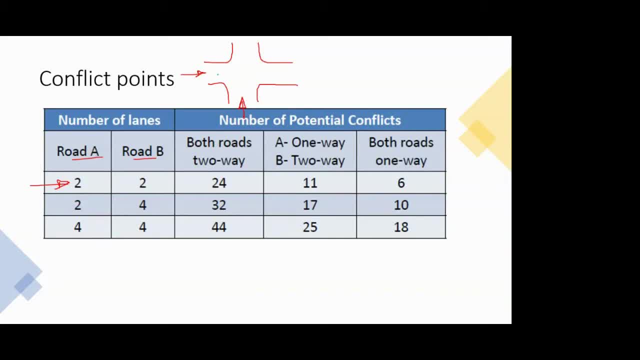 The movements. Suppose both the roads are two way, Two way Two lane roads, So that two way traffic is allowed on that road. I will just draw the center line So that it is clear to you. Okay, And now, if I go on drawing the movement, 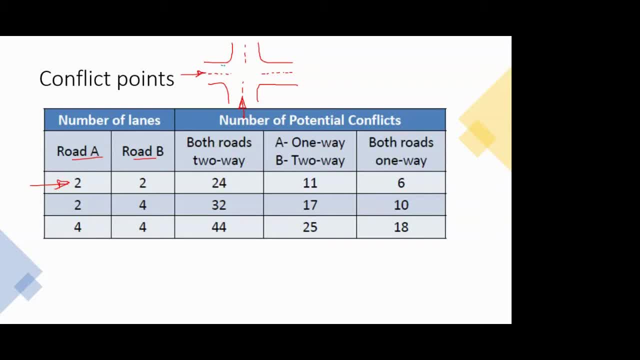 So, coming from this direction, My vehicle, It can take a turn to the left, It can go straight Or it can go right, Considering we are seeing the scenario of Indian traffic. So that is why left hand drive. So, similarly, if I go on plotting, 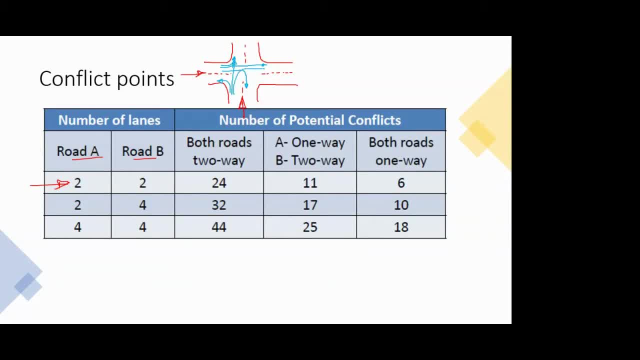 I can have a little more of this. The public road. So now, as a space is limited, If I draw all the movements So it will be sort of congested And then I will not get to know what I am trying to say. 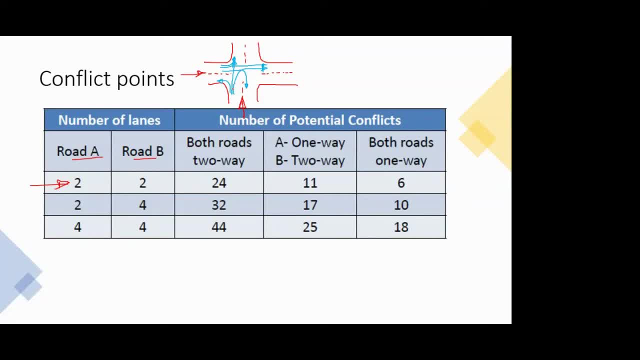 So I will just draw this. two movements, Okay. Now, wherever you see there is an intersection between the two lines. So those are nothing but the conflict points. Okay, so the more conflict points, more susceptible that intersection is to a accident, if you are not. 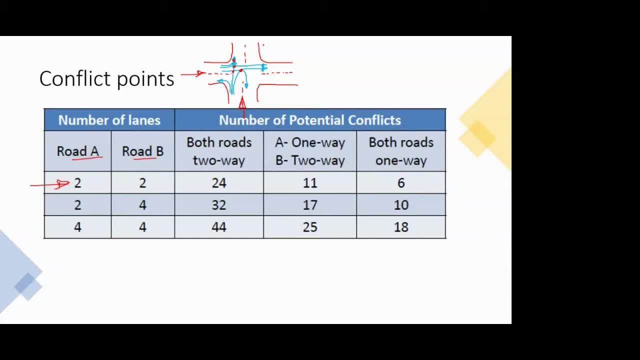 providing any control devices. control devices, as in you, are not providing any signals or not providing any islands, channelizing islands. so in that case, this conflict points goes, goes on increasing. okay, so you can see here, in a two lane road, when two roads are having two lanes, 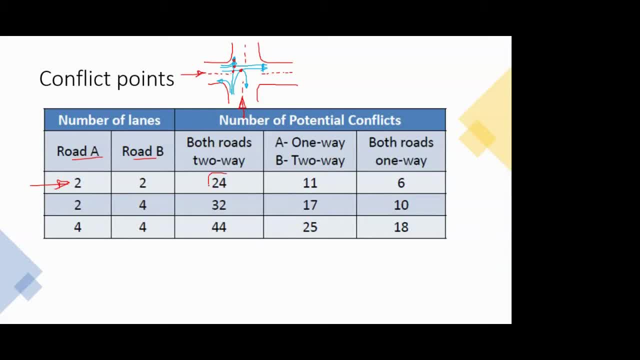 and both are both roads are two ways, so the conflict points are 24. but the moment we make one road as one way and another road as two way, the conflict points reduce drastically. and if we make both the roads one way, so the conflict points reduce even more. 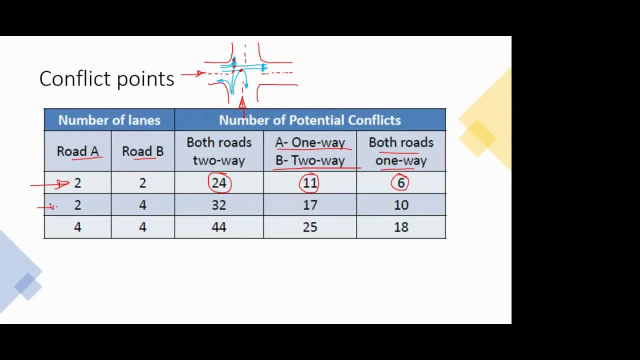 similarly, i have given the scenarios. if you have two lane, four lane and a four lane, four lane combination, okay, it's okay. so what i had i want to show you is these values: see the decrease in the values. so what you can see here is when you have a one-way, one-way street. so the number of conflict points they reduce drastically. 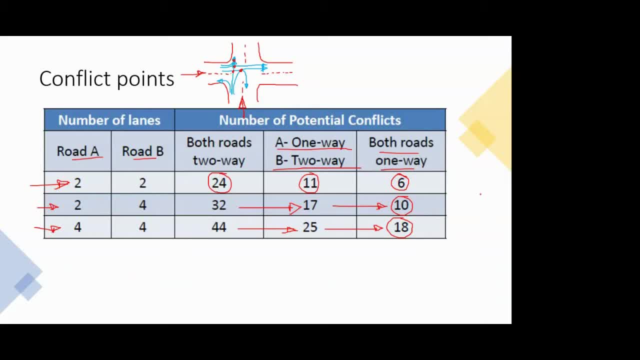 and that's also one of the reasons that- and if you are staying in a metropolitan city or any city which is having a fairly congested traffic, so after some point of time they might have converted a couple of- uh main streets in your city into a one-way, and the reason for that is when you 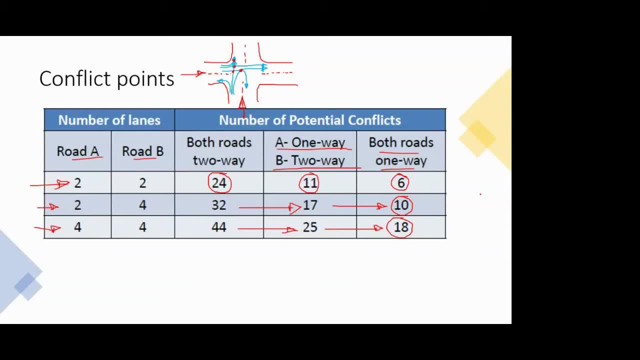 make it a one-way, then the conflict points reduce and then the intersecting or the crossing maneuver gets reduced. and if the crossing maneuver is reduced, then automatically the delay is reduced, the speed increases and then you get a free flowing, or even if not free flowing but a fairly moving traffic. so always remember for a traffic engineer. 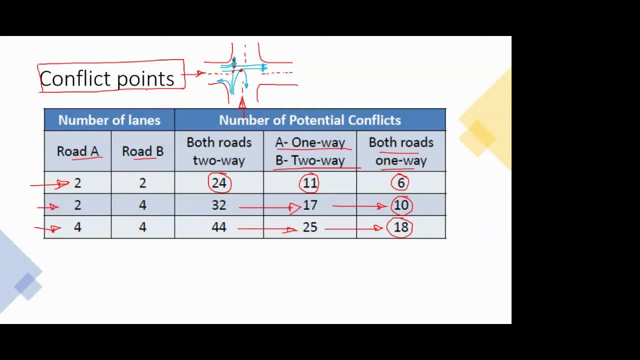 Reducing this conflict points is a very tricky job, or can say a challenging one, because he or she has to reduce this conflict points without affecting the level of service of the road. So, in order to reduce conflict points, it should not happen that you are making the 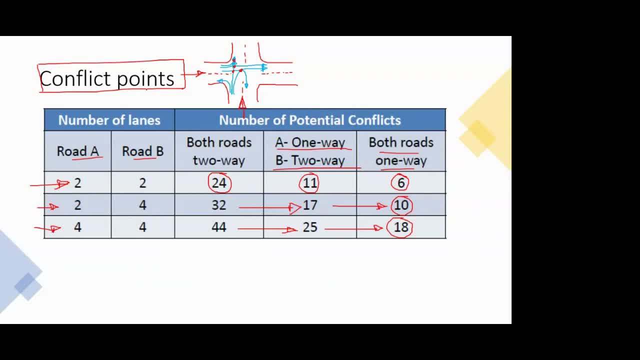 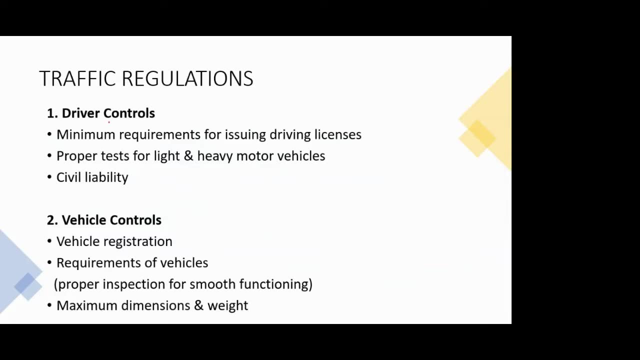 driver to go ahead further two or three kilometers and then take the desired turn. So in that case also, the drivers will not follow this and then there will be breaking of the rules. So this is related to conflict points. Now, as far as the traffic regulations is concerned- now, you have always heard of these terms: rules- 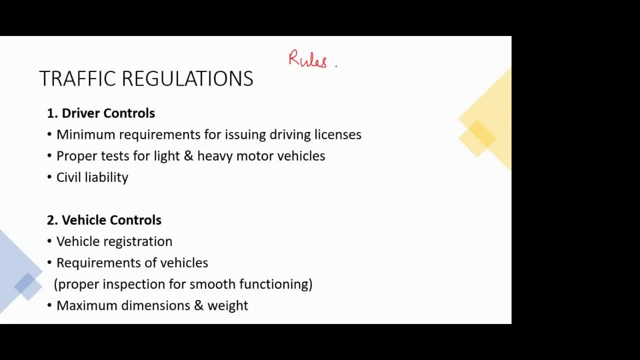 and regulations. I hope- and I am sure not hope, I am sure that everybody must have heard these two terms at some point of time in their life- that you should follow rules and regulations. So, just before starting this traffic regulation, if I have to tell the difference between: 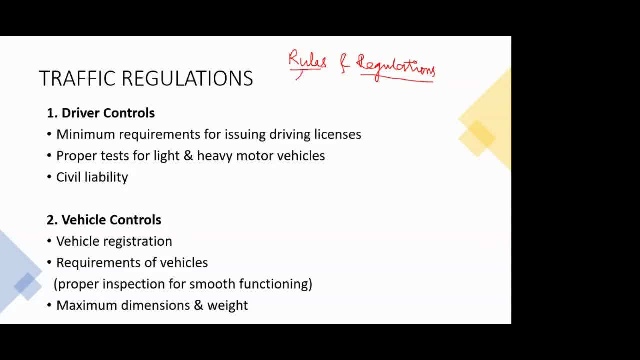 these two. so the difference is rules is something that they are sort of a guidelines. There are guidelines so that all the things in that systems or in the particular system they go on smoothly. So as far as the traffic is concerned, so there is something called traffic rules, which 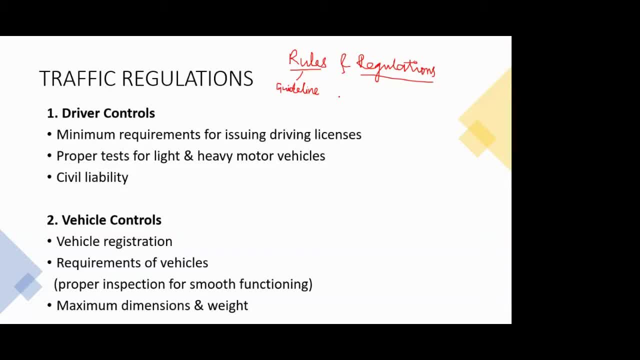 are More of a guidelines. So if you follow those guidelines, your traffic stream will be efficient enough. And regulation is something when these guidelines are abided or you make a law behind it. Suppose overspeeding, so you should not drive at a on a road. 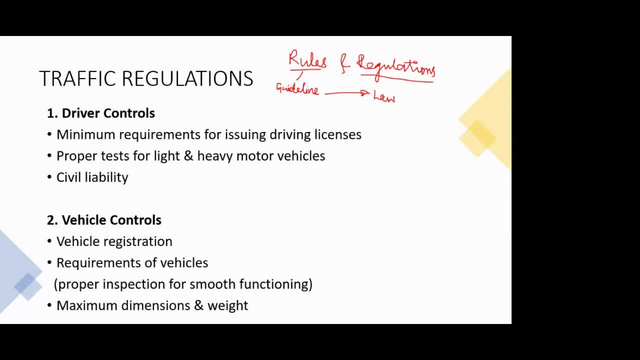 Suppose there is such statement that for a particular road, you should not exceed the speed of your vehicle above 80 kmph. So this is a rule. But when you stick a law to it that if you do so, if you go above 80 kmph, then you will. 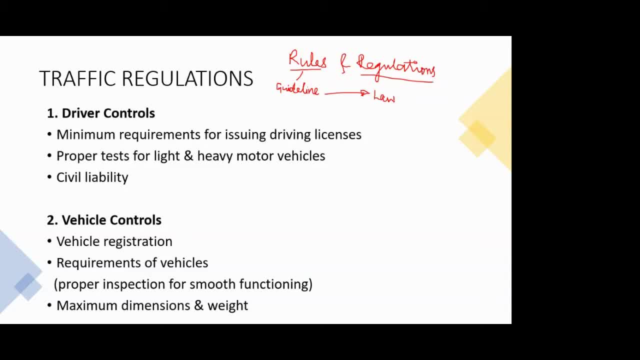 be fined 1000 rupees, So that becomes a regulation. or if you are drinking and driving, or you should not drink and drive, That's a rule. But if you drink and drive and you get caught, then you are liable to a regulation. 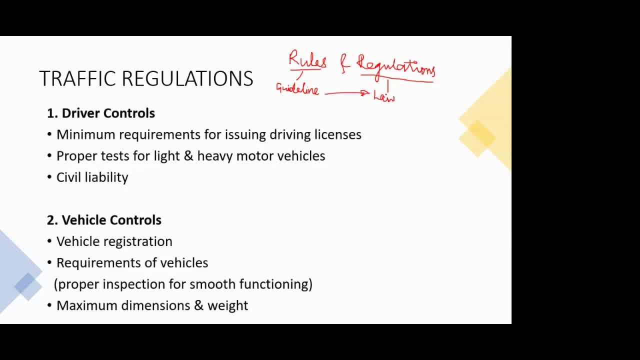 So that becomes a regulation, So that becomes a regulation. or if you are drinking and driving, or you should not drink and drive, That's a rule, So that becomes a regulation. So that becomes a regulation, So that becomes a regulation. So in that case what we have done is we have attached a law to a particular rule and then 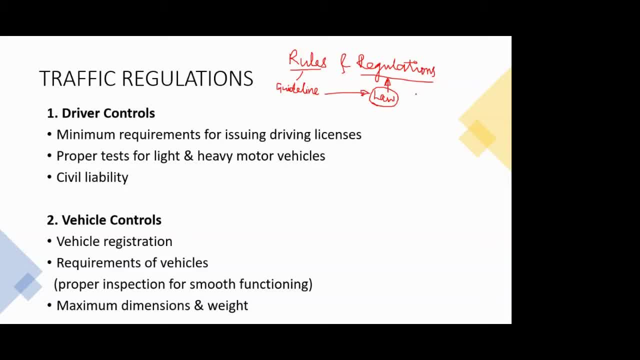 that becomes a regulation. So this is the main difference between rule and regulation. Rules are specifically guidelines which, if followed, everything in the system goes on smoothly. But regulation is when you attach a law to that rule, Okay, And then you enforce that. 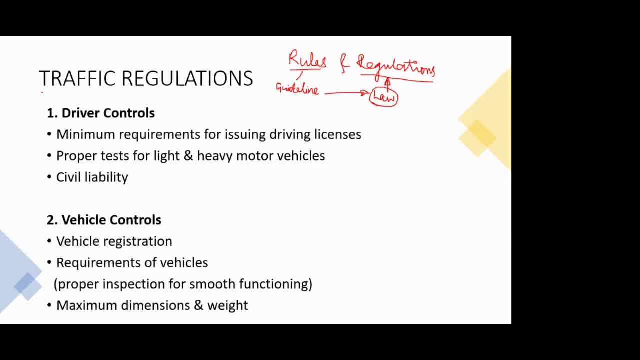 that law, then it becomes a regulation. so from our traffic point of view, you all know that there are traffic regulations. now you know the difference between rules and regulations. so next time, just whenever you get a chance, go through the motor vehicle act, which has been revised recently in. 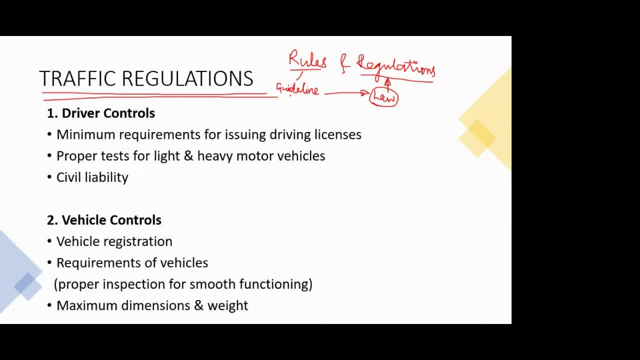 couple of years. so in that you will get to know what are the rules and what are the actual regulations. okay, so regulations. they can be divided into four different category. so first is driver controls, that is, such regulations which will control the behavior of the driver or the 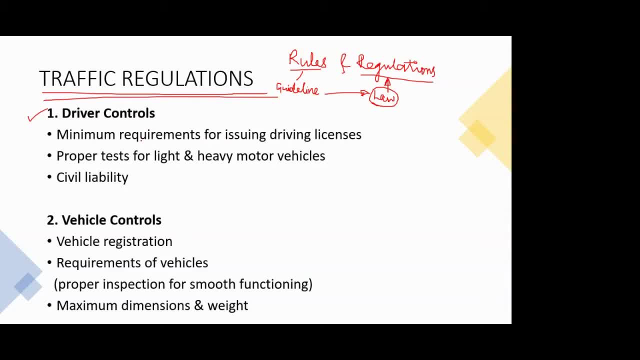 movement made by the driver so that or those driver controls or traffic regulations related to driver controls. they include regulations such as the minimum requirement for issuing driving licenses, that you should be of this much age. you should pass that much that test. okay, so all that thing, then proper test for lcv and heavy motor vehicle and then civil liability. so these are the. 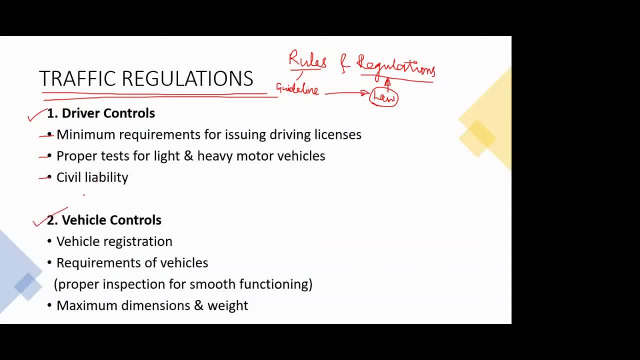 regulations under traffic controls, under vehicle controls. these are the regulations which are a mandate for a vehicle and mainly it is vehicle registration, the requirements that it should be in a proper working condition and the maximum dimensions and weight. so many of the times you will not. you are operating around a vehicle in a vehicle, but when you inform, that comes to your. 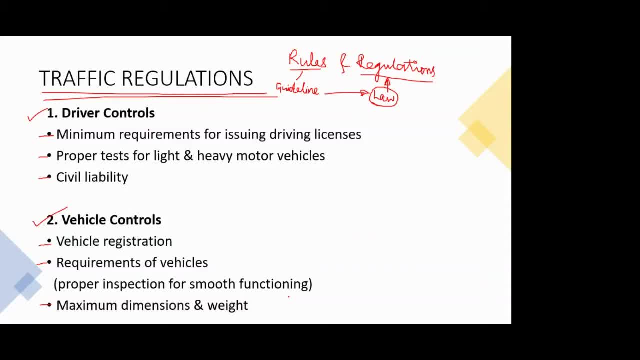 reference to a vehicle, you have to identify it that it is not a vehicle, not in an individual vehicle. that is a vehicle. now, one of the things that we have done is that we have been able to determine that the vehicle does not come anywhere in the vehicle, because if someone is driving, 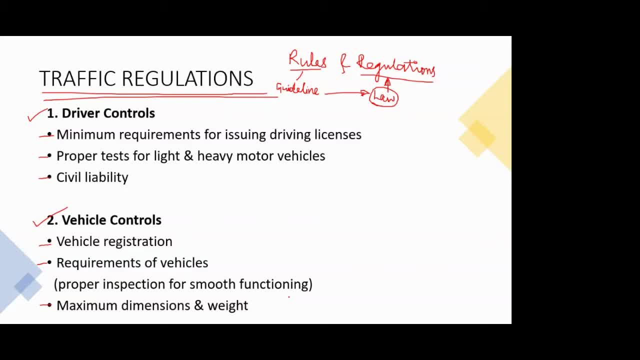 on a vehicle, then we have to build a vehicle on that vehicle, so we have to build a vehicle for that. so this is one of the reasons why there is no limit on what skeleton or a body we can mount over a chassis of a truck. if you have seen a new truck, a brand new truck, 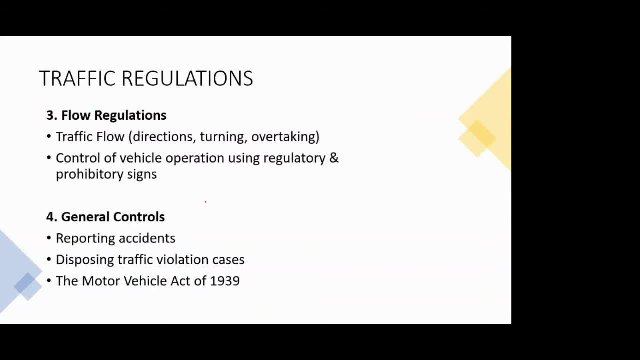 so it doesn't come with all that cage kind of thing. so a truck just comes with the engine, the main cabin and traffic regulation then related to flow control, as in to control the movement of the vehicle on road. then you have regulations such as you have a direction regulation that you have to only follow. 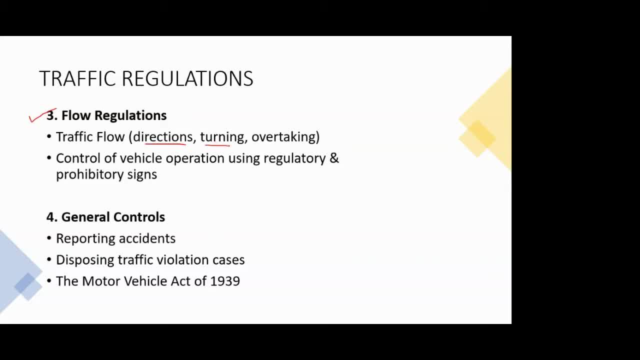 one-way traffic or two-way traffic, okay, right turn not allowed, then overtaking not allowed, and such kind of things. and also in flow regulations, you have this control of vehicle operation using regulatory signs so to in order to enforce all these things, then the signage is are installed. 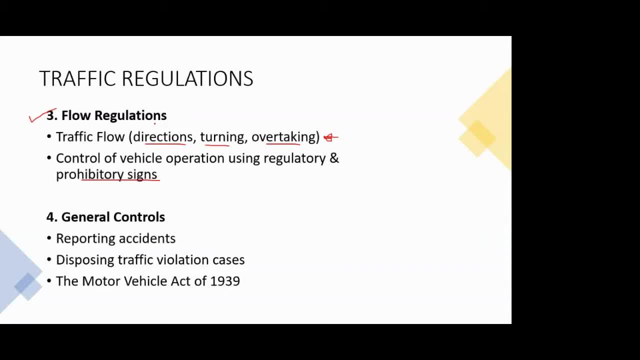 and if you violate them, then you are subjected to a fine or any legal action. and then fourth category is general controls. now, these are related to the control of the vehicle on the road, and if you talk in riders, ok, Musik way and then down, you will get all these furtherller. that also. 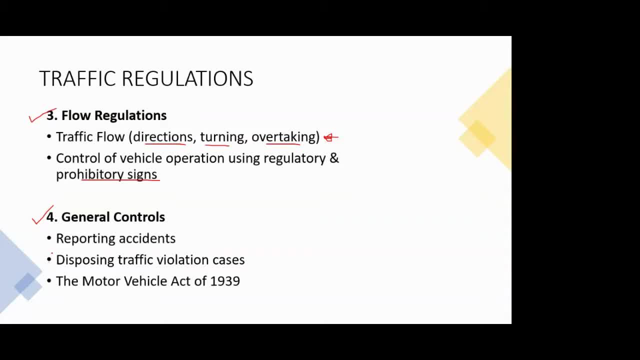 are related to, like reporting an accident or disposing traffic violation cases and all this what I have mentioned here. so this motor vehicle act- now you have- I have written the first version of it, but it has been recently amended, I guess in 2016, 2019, somewhere in that period. so if you, 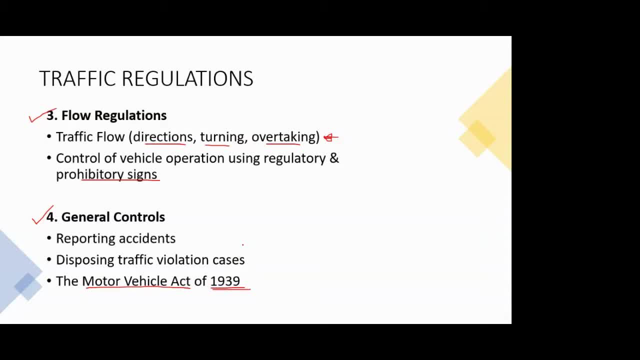 get a time and if you are interested, you can just go through this Motor Vehicle Act and You'll get through this Motor Vehicle Act and you'll get to know that, to know some more rules, or you might also be surprised to know that what are the rules and? 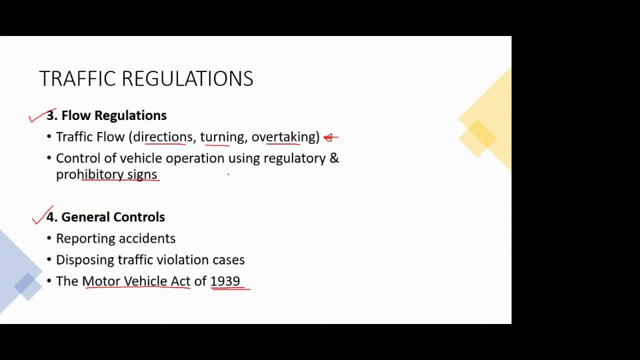 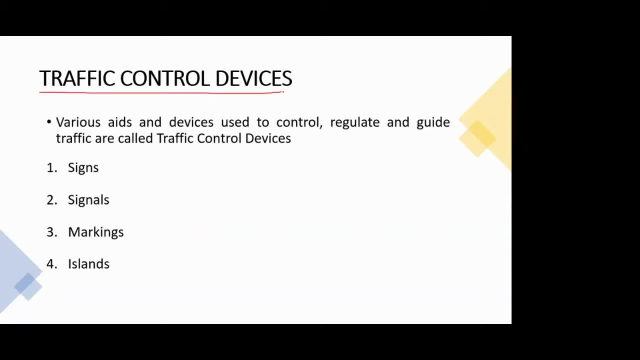 what are the actual regulations? so this is regarding traffic regulations. now coming to the main discussion for today is traffic control devices. now we are saying that traffic it includes vehicles and people and pedestrian, vehicle passenger drivers and pedestrian, so it's of a dynamic nature. we have seen in the traffic characteristics also that 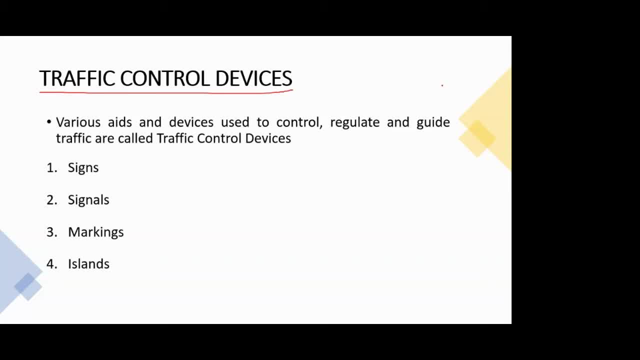 road user characteristics. you have a lot of load user characteristics like vision, hearing, reaction time and environmental factor, mental factor, psychological pattern, all kind of branches you have seen. so if you have so much variation on any road, so how to control this traffic? because it's not like if you? 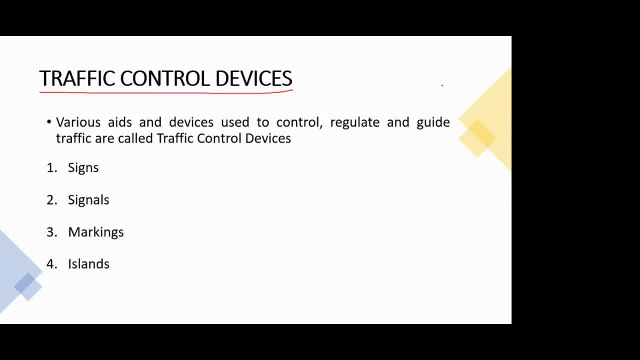 come up with some regulations, everyone is going to follow it. okay, and instead of making a regulation for each and everything, it's also very tedious to keep a track now for each and every movement. if you go on applying a law, so it will be tedious from the enforcement point of view also. 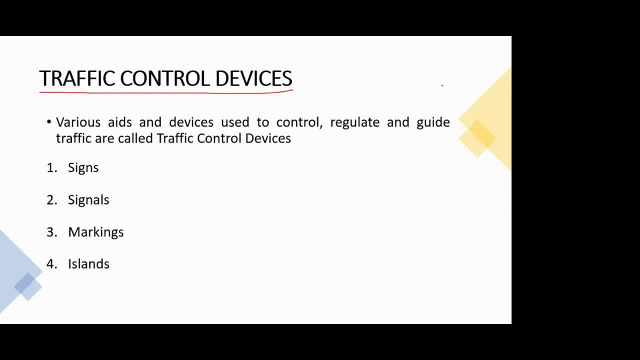 that the traffic police itself will get confused that what is the law for which violation? okay, so for that, you need to do something in order to control this traffic, without or with using the minimum regulations. so for that, we have this for our help, that is, traffic control devices. now, though, the word is devices. when you, we will look. 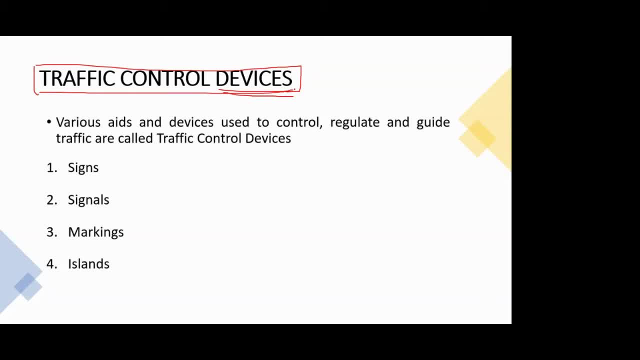 into what goes into this, you will actually come to know that it's not actually a device or a mechanical working thing- it's not like that, okay- but it is something more of a stationary kind of stationary kind of thing, but it acts as a guiding tool for the traffic to go in a particular way. 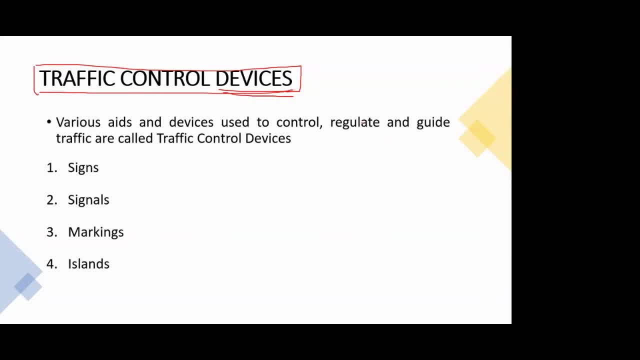 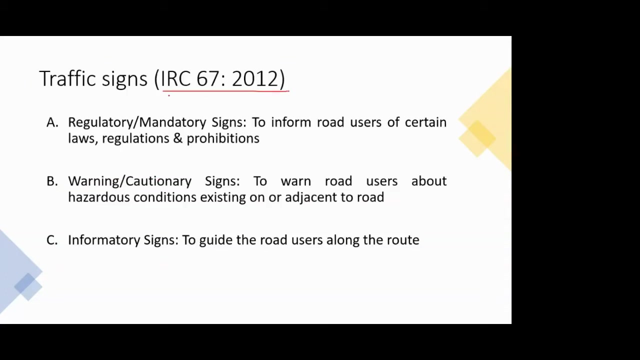 or move in a particular direction. so in traffic control devices you have these four devices that are predominant, these signs, traffic signs, traffic signals, traffic markings and traffic islands. so we'll see one by one. in brief, so related to traffic signs, now i have mentioned an irc code, so obviously i can't cover everything in one particular lecture because each of this 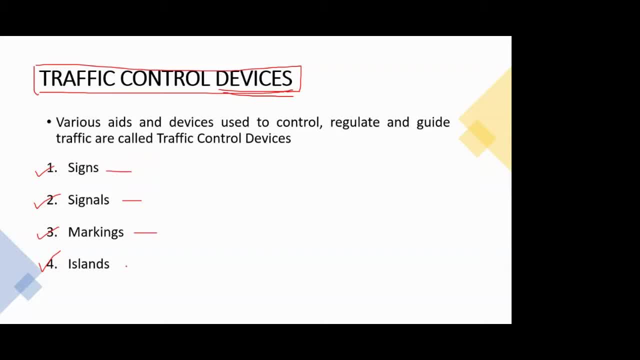 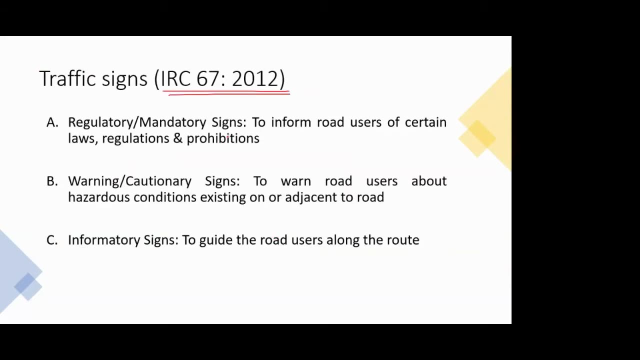 traffic control devices has a different code for it, and each code is of hundreds and or at least 100 or 50 pages. so i can't cover everything, so that's why i have mentioned it here. so it's up to you. you can go into detail at your end. i'll just give you the short summary of it. so, in traffic, 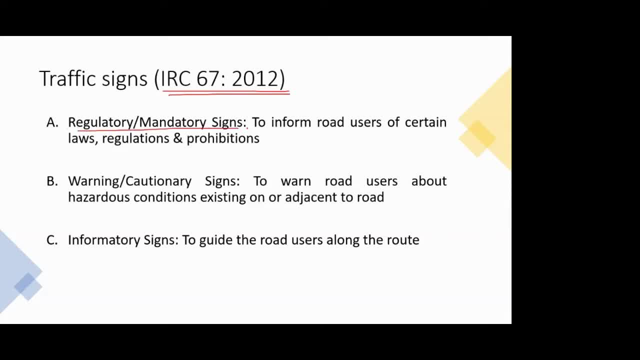 signs you have mainly three types. one is the regulatory, or mandatory signs. second is the warning, cautionary sign and third is the informatory. so a regulatory is this. now you know what a regulation is. okay, so regulatory signs will be something which tells you about a law. okay, so mainly they are the prohibitions and all kind of. 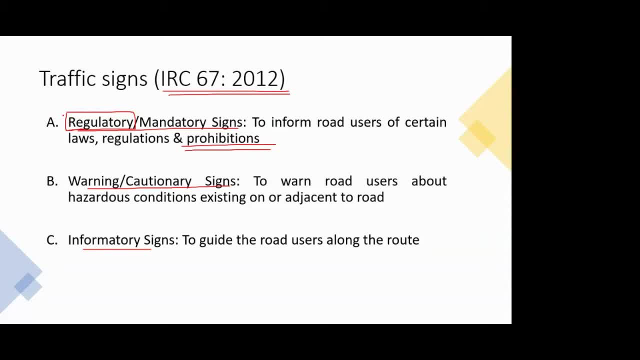 thing. so if you do not follow these signs, if you do not follow the regulatory signs, then you are bound to get a legal action upon you or you will be subjected to some fine. so you need to know what is a regulatory sign at first. we'll come to that later. then, b type: you have a warning sign, or 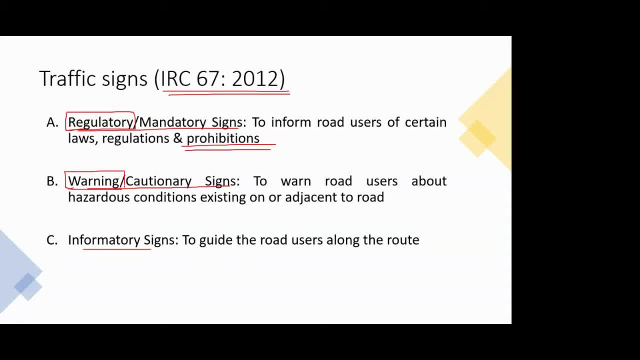 cautionary sign. now, this is a warning sign, and this is a cautionary sign and this is a warning sign. this will not or violating these signs, they will not give you a fine or any kind of action, but they are just for your information so that you don't end up with some accident. okay, 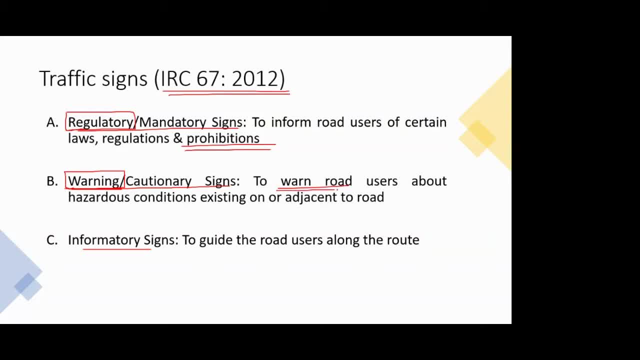 so it is just for the road users to warn about something. okay, maybe there is an ongoing activity on the road or there is a height restriction, okay. so those are something warning or cautionary sign. and then there is something called informatory signs. now, these signs have absolutely nothing to. 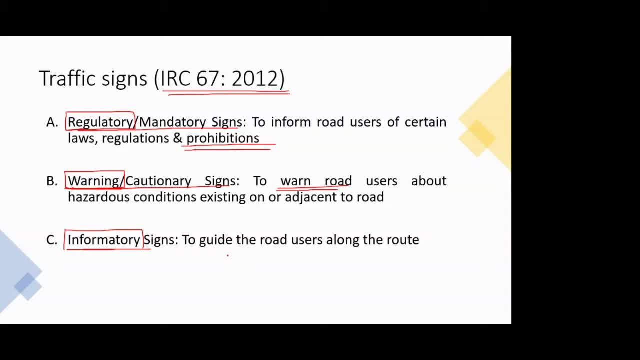 do with the regulation nor the warning, but they are just for information. like 250 kilometers, there is a tunnel thousand meter ahead, or there is a toll booth one kilometer ahead. so all these are informatory signs, okay, so now we'll quickly have a look on it. so first is the mandatory descent, now 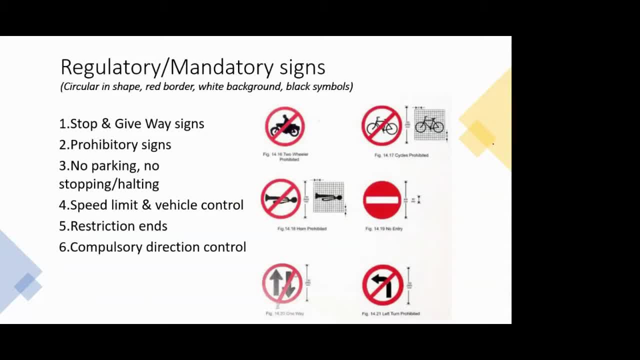 as i told you, if you violate these mandatory signs or regulatory signs, then you are subjected or you are liable to a fine or a legal action. so how to actually make out or how to identify that which sign is a mandatory sign or regulatory sign and which is the other two categories? so they have come up with. or in india, they have come up with. 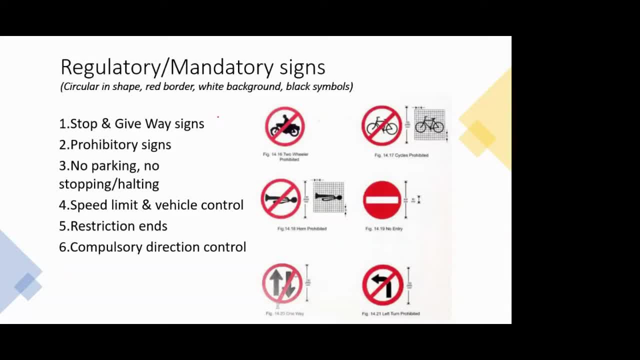 a pretty, very good, straightforward way for the classification that the regulatory sign or mandatory signs. it will always be in circular in shape, always. okay. it will always have a red border with a white background and whatever they have to write inside it that will be in black color. this is the standard one, because i told you that. 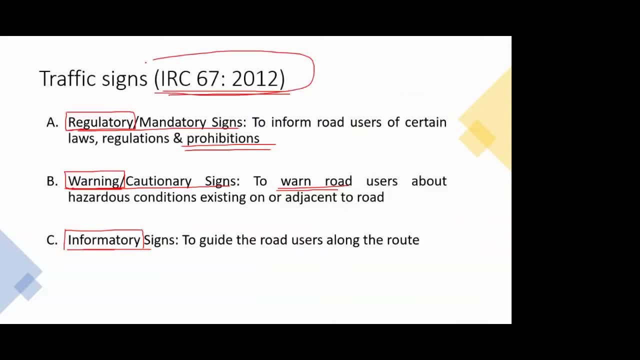 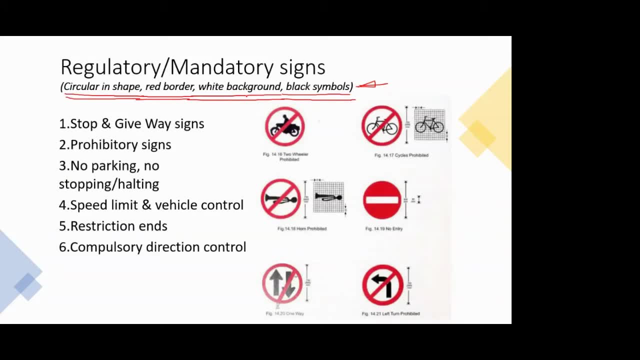 you have a irc code for all these signs, so whenever any traffic facility is being constructed. so in the design aspect you have some miscellaneous design and in that this signage design also comes into picture. okay, so always they will follow this mandate, or rather they have to follow. if they don't, so it's wrong on the part of the. 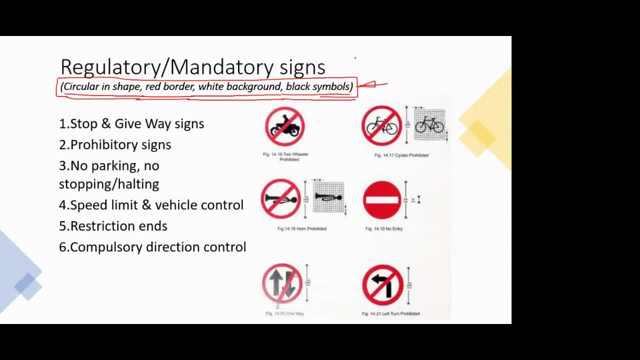 authority who has built that road? okay, so regulatory or mandatory signs always circular in shape: red border, white background and black symbols. and, as i told you, you can't violate this, not what did this, rather, and if you violate, then obviously you are subjected to some finer legal action. so some of them i have listed here now. these are not. 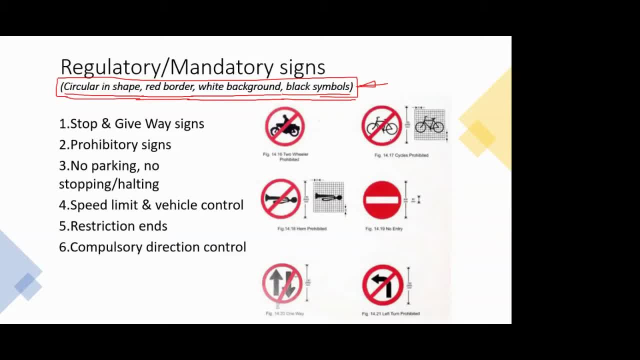 the complete list or the figure on the right. also, i have not shown all the signs, because there are a lot of them. so just for educational purpose or just for sake of going through all the signs, you can open that irc code and then you can just have a. 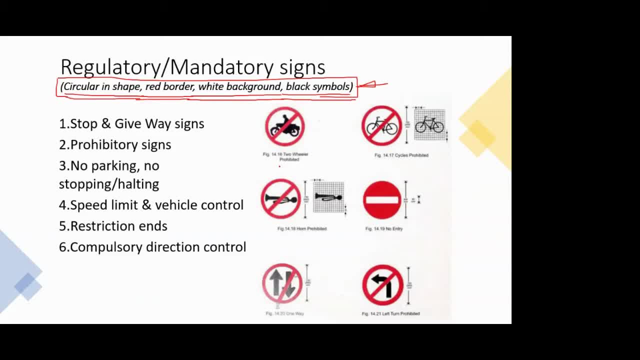 look on all of them. no need to buy, had them or not to study from the point of view of any exam, but just for your information that at least you should be aware while driving or even while walking, what are the signs that you should follow. so some of them are. i have listed here: stop and. 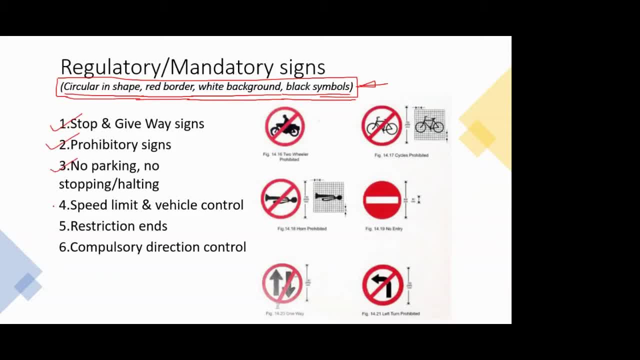 give way sign, prohibit, resign. no parking, no halting speed limit. this is also one of the most neglected uh signs in india. the restriction ends compulsory direction control. as in uh you are, compulsory direction control is uh one way or a left hand prohibited, that kind of thing. 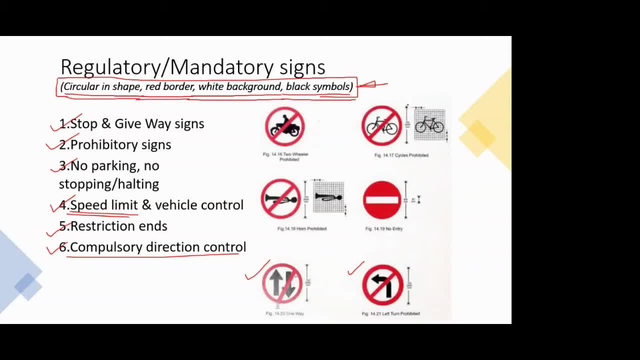 so on the right side, you, if you see the figures i have shown you, and now you can see something written over here. so they have also specified what should be a size and even what should be the size of the font inside it. so everything is given in detail. you can just go through it, for. 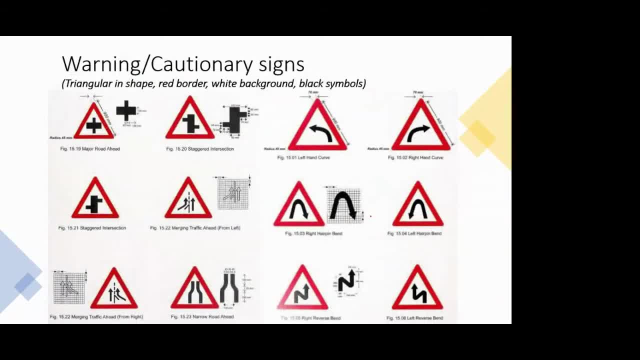 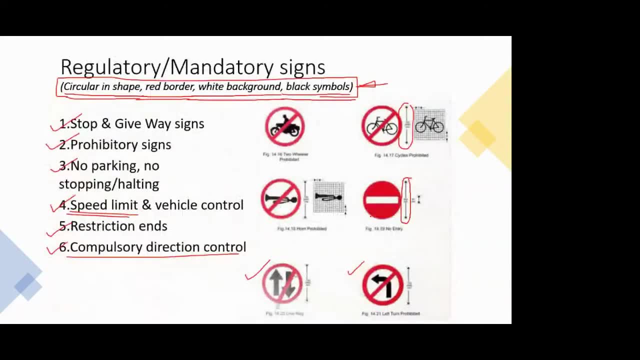 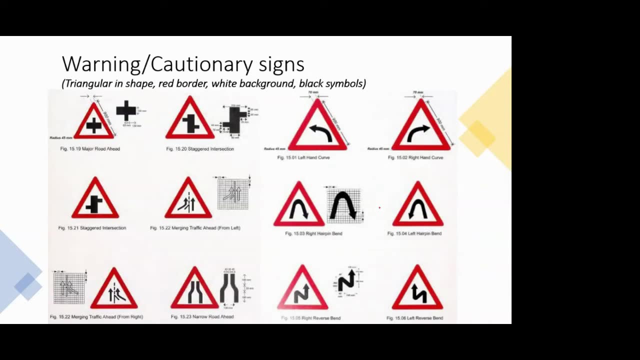 information purpose. then comes the warning sign. main difference between regulatory and warning: you can see it very drastically in the picture itself. so this is regulatory and this is warning. so the main difference is regulatory is circular in shape and warning is triangular in shape. rest: all things are same, just the shape changes. that 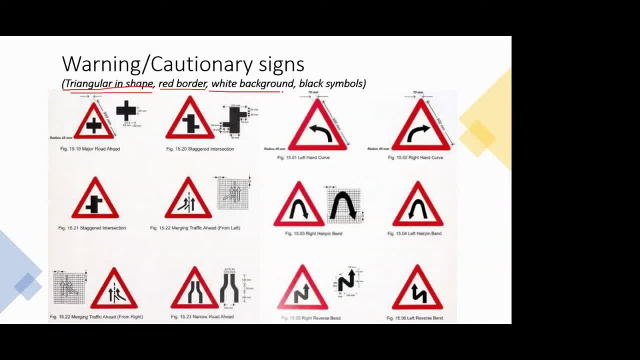 it's triangular in shape. rest of the things, like red border, white background and black symbols, they remain the same and, as i told you, it's just cautioned or sort of a warning to the driver or the road user. like a major road ahead, or you have a left hand curve or a right hand curve. 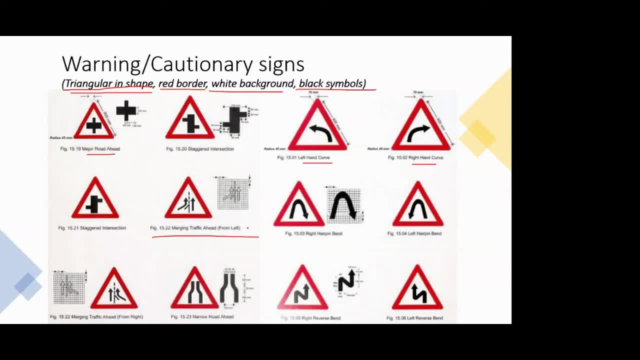 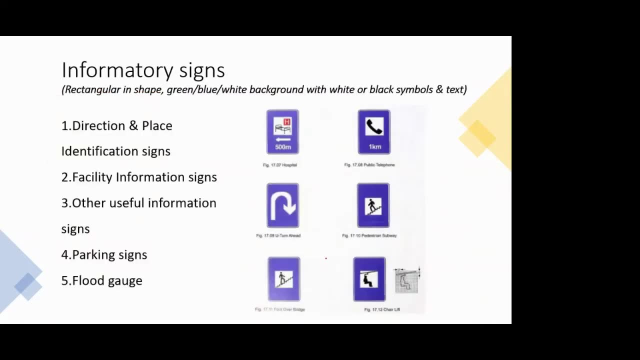 or you have a merging traffic ahead. so these are some warnings to the driver. or in the hilly roads, you must have seen the sign that there is a s curve or there's a steep, uh gradient ahead. so those are the warning signs. and then you have informatory signs, as i told you. they are just for the information, and some of them 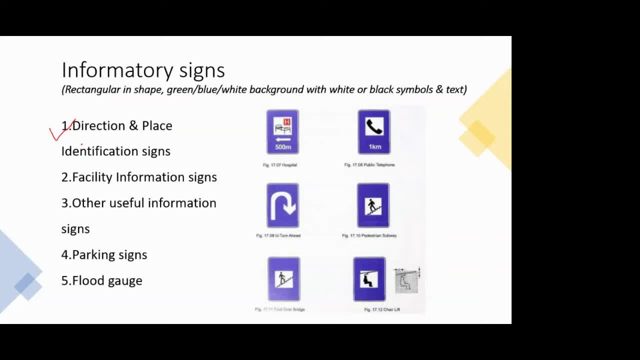 i told you that, that you just for the information, that you, as you know, the information is just there for the information and some of them i told you that the direction and place identification sign that left road will go to pune, straight road will go to, suppose, mumbai and then something else. so like that kind of thing then, other than that you have. 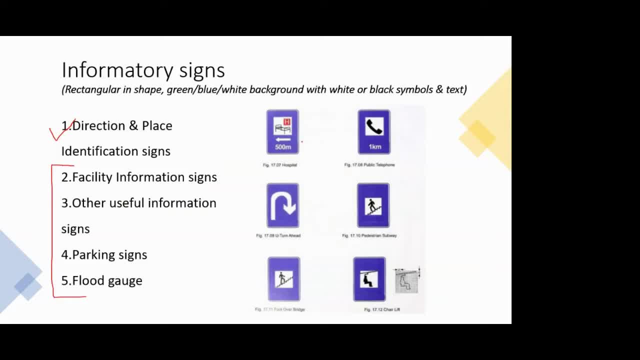 these that different facility information, like there is a hospital, there is a public telephone, there is a pedestrian subway. so these kind of signs come under informatory and if you see the visual characteristics of this sign, so they are rectangular in shape, they are either green, green, blue or white background. so this is the variation that they can have and the symbol also they can. 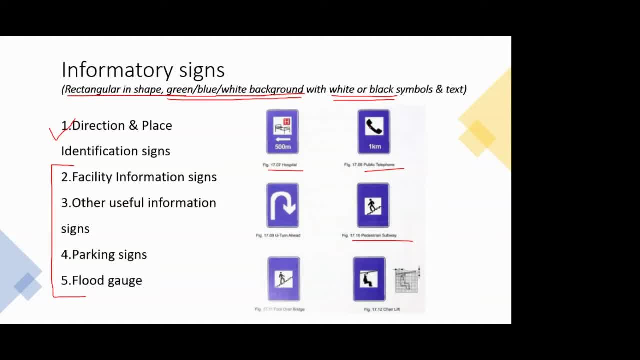 have white or black. so, other than red, all the colors are used in this informatory site. so these are the different traffic signs and this is one of the traffic control devices. so, looking at these signs, it is sort of understood that the road user, whether it's a pedestrian, whether it's a truck driver, 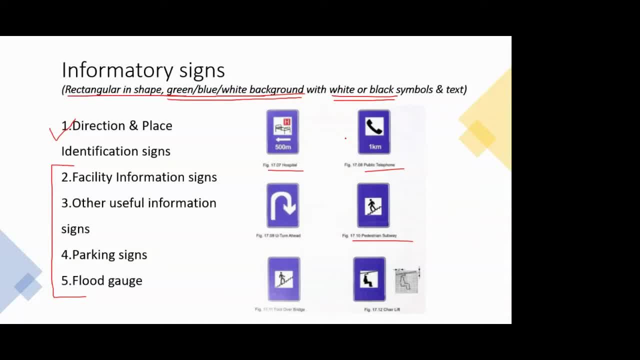 or two-wheeler driver, or even a cycle cyclist, so that person will look at these signs and then he or she will change the way if his he or she is not traveling properly or not moving in the proper way on the road, so they will change their course accordingly. 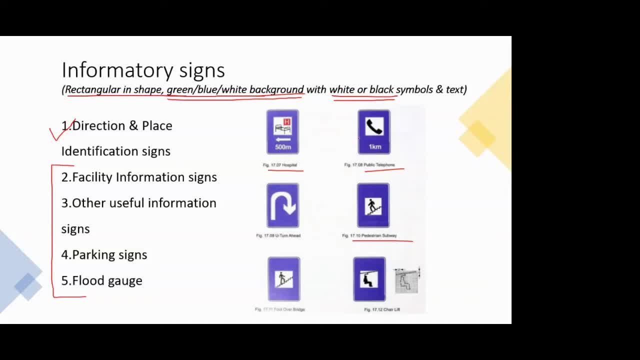 okay, so that's why it's under traffic control devices. now, as i told you, these are not actual devices, so you can also see them. so these are just stationary signs. okay, so there is no working mechanism, mechanical devices or such kind of thing. but then to their term. 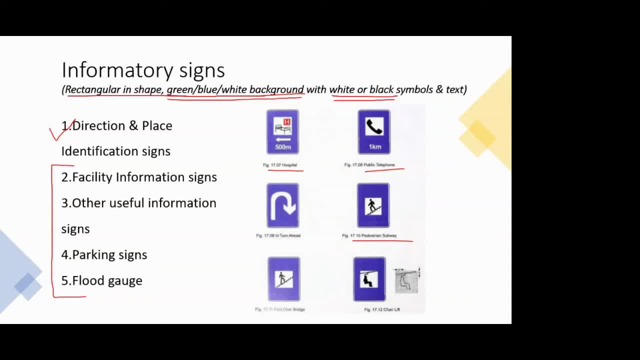 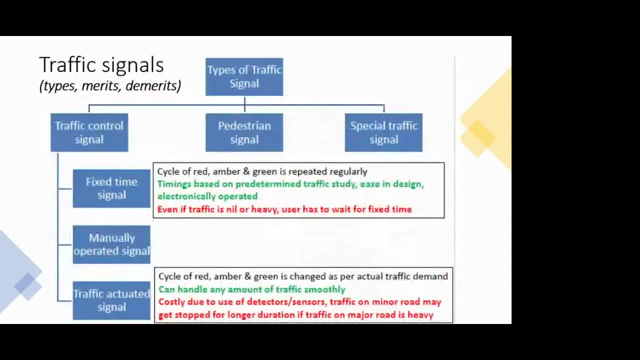 devices because they do the work of controlling the movement of your vehicle, okay, and to some sort, the behavior of your driver as well. then the next traffic control device is the traffic signals. now again, this you all must have seen. i'm very sure at some point of time you have seen what are traffic signals. but what i'm going to just 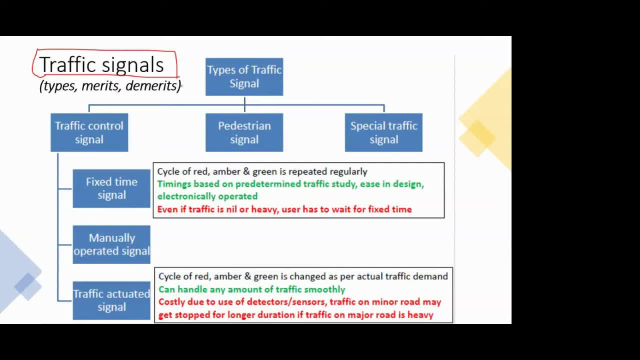 show you is a short classification of these traffic signals. so one is traffic control signal, one is the pedestrian signal, which is exclusively for pedestrian. this also you must have seen on the crosswalks, okay, and then you have a special traffic signal. special traffic signal as in: 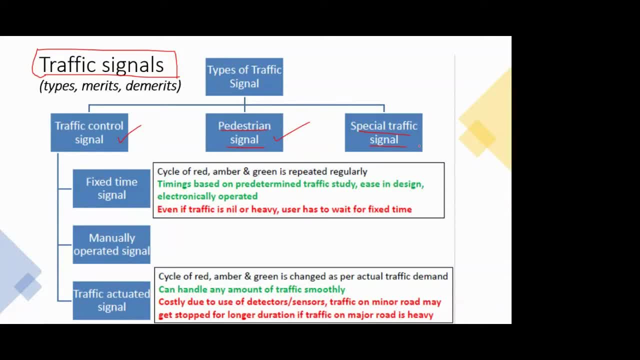 it's a specially designed traffic signal for, suppose, only a taxi lane, or only an ambulance lane, or, in some cases, if you have gone through any military area. okay, if now let's assume you all have traveled somewhere in the pune city. so you know, in pune city you have three to four cantonment areas, that is military area. 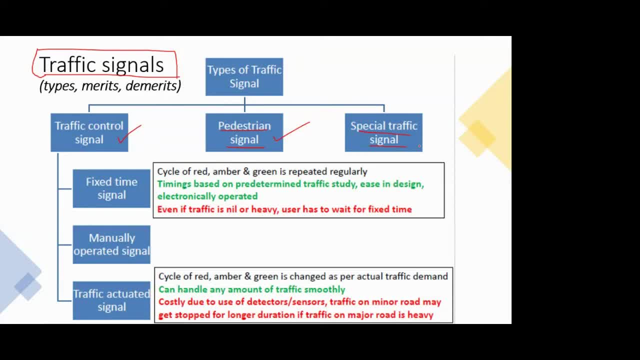 dehu road in pcmc khadki, then in pune you have pune cantonment. so when you go through these roads, at some points there are traffic signals which are not needed, but they are still installed because they are the special traffic signal. the best example i can give is: 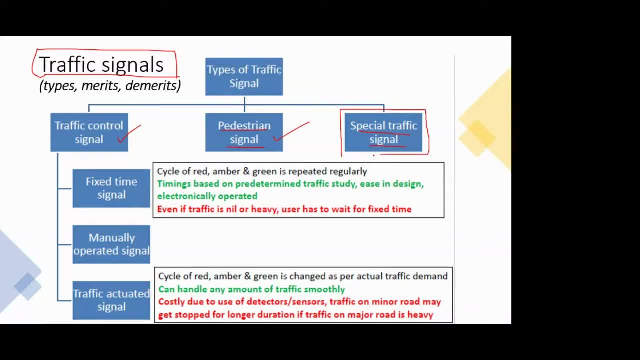 the college of military engineering, cme, which you have in dapoli between dapody and khadki, so there it's not an intersection. also, next time, whenever you go, you just see to it it's a straight road, okay. and on the left hand side, if you are going from mumbai or if you are going from 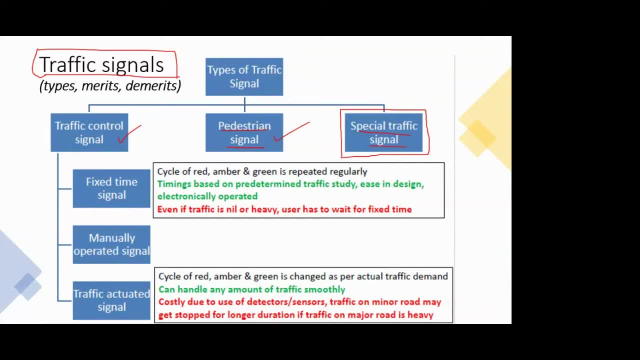 pimpre towards pune. so on the left hand side you get the main gate of cme and it's a straight road. there is no right turn or nothing like that, but there is a tripraft community of four to five days, which means at least you go to that state road and then when you go back by the road, 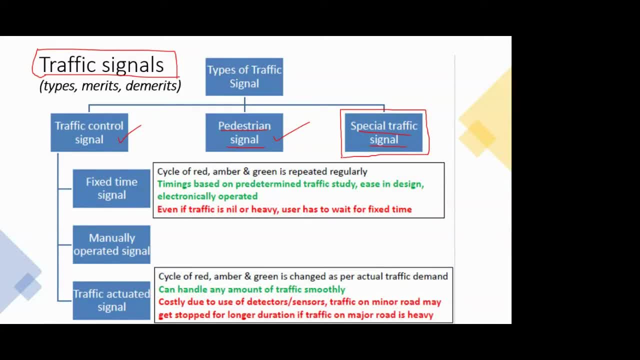 there is a or the tram of that you have. in that, though, that you have to go to that street, which is of 10 degrees. there's no traffic signal that, but there is a gate of cme on left side, so that's why they have installed a traffic signal. 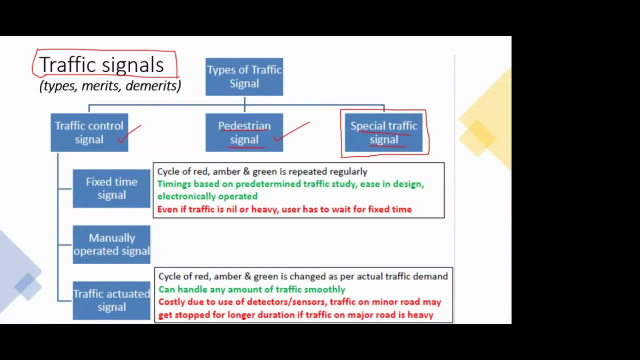 over there and that is a special tribe, that it suppose there is a higher authority vehicle or a person who from military having a higher force, so that person is traveling and then he is entering or leaving cme, so the signal will be controlled by someone sitting near the gate. 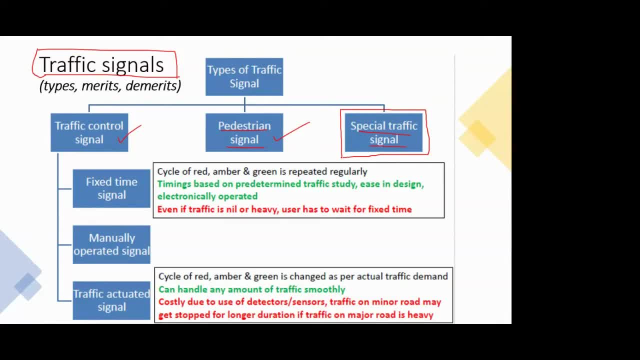 of cme and then they will give way to that special or vip vehicle. so that's a special traffic vehicle. these are very rare to be seen. you can see it at such location, one such traffic signal. another example i can give is in delhi, the crri- now this you have heard- determined first unit. 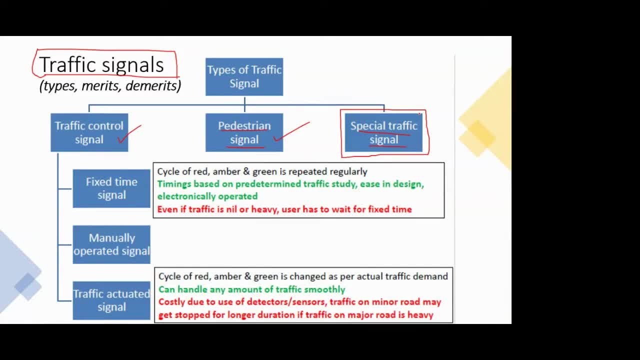 central road research institute, crri, which was one of the outcome of jaikar committee. so in new delhi you have headquarters of this crri and there the same thing is there that it's a main gate of crri and it's a straight road. but then too they have a traffic signal over there only because the 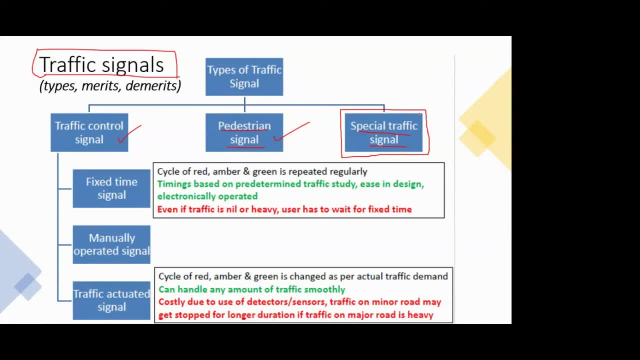 vehicles which are coming out of that institute are going into that institute, so they control the signal likewise. so that's the special traffic signal, now coming to the our regular traffic signals that we see in everyday life. so they can be categorized in three types. one is the fixed time signal, in which, whatever is the cycle of your red, amber and green time, so it is. 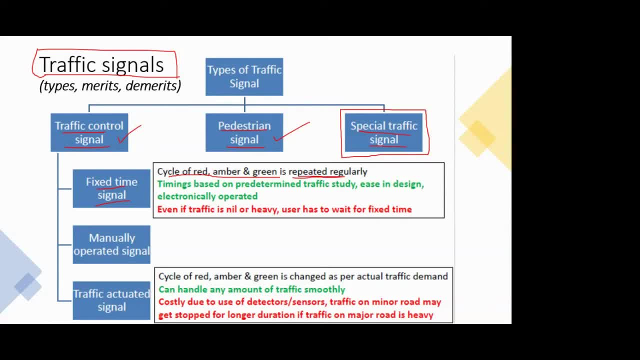 fixed and it is repeated regularly, so there is no change. if it's a 60 second red, two seconds amber and then 45 seconds green, so this will be the cycle which will be repeated throughout its life, until until, until, unless it is changed. okay, then you have manually operated. 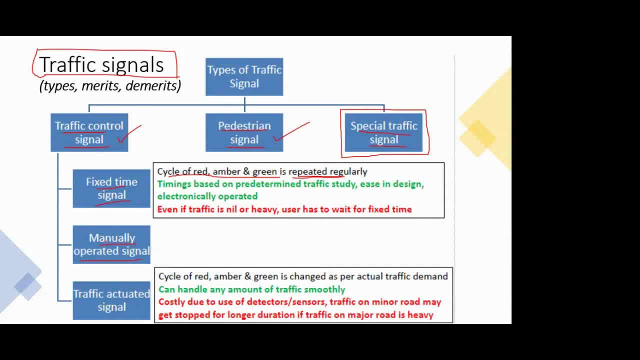 signals, now manually operated, is from the name itself, you will see. so there is no fixed duration as such for any cycle- a red cycle, green cycle or amber right now- but it is controlled by the person who is sitting over there, so sort of you can say that even if there is not a traffic signal and you have a traffic police. 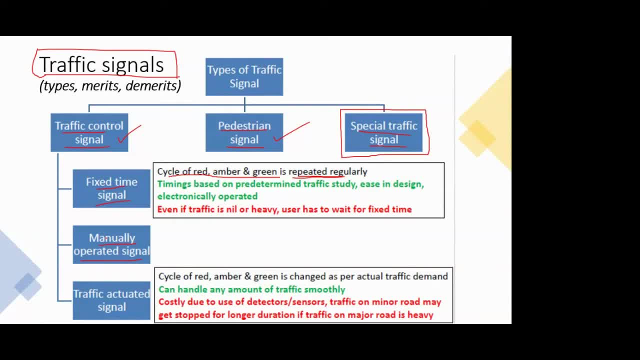 at a particular intersection, so that traffic police also controls the movement of the vehicles without having a traffic signal for itself. okay, so that is the way manually operated signal works. and then you have traffic actuated signals, which are a pretty sophisticated development in this. traffic signals that, whatever is the cycle time, 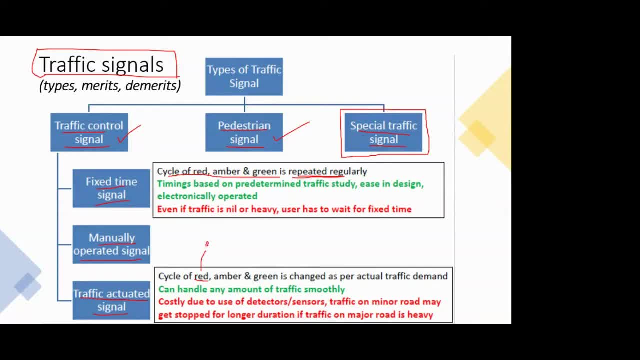 now, whatever example i gave, that red suppose it is 30 seconds, amber is 2 seconds and green is 45 seconds. so this will hold true for a particular traffic scenario. but now let's say that at night time, you all know, at night time the traffic in the city roads it reduces drastically. 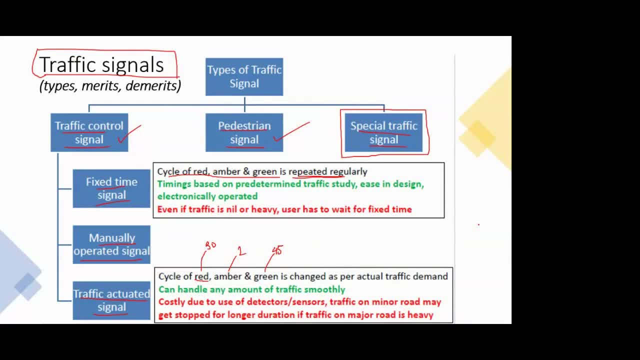 so suppose there is a road, or many of the times you might have also wondered that the road is empty, but still there is a red color signal or the red light is on and that signal is working and you have to follow it. by regulation you don't follow it, that's another thing, but you have to follow it. 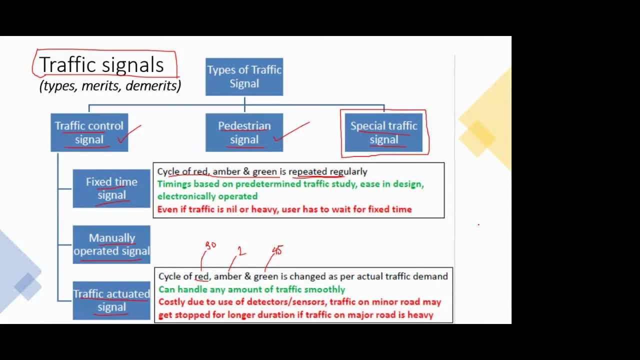 but it doesn't make sense. that a sense that the road is empty. there is no vehicle on it except your vehicle. so why to stop there? so your argument is correct, and there you can have such actuated traffic signals. so what these do is cameras are installed with different perspectives. okay, so 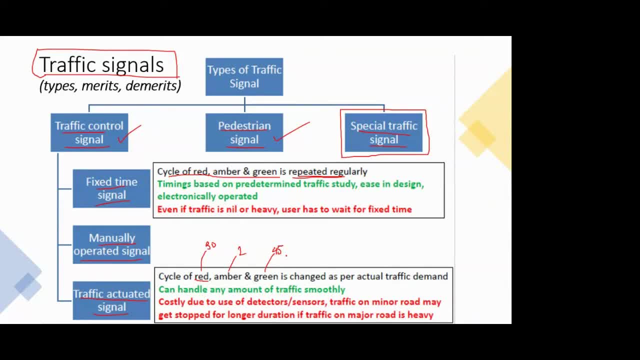 that different views are seen of all the roads and all the vehicles coming towards that intersection. and then sensors are installed so that the traffic or the movement of the vehicle is counted. okay, so what we have seen in classified traffic volume count. i told you that there is. 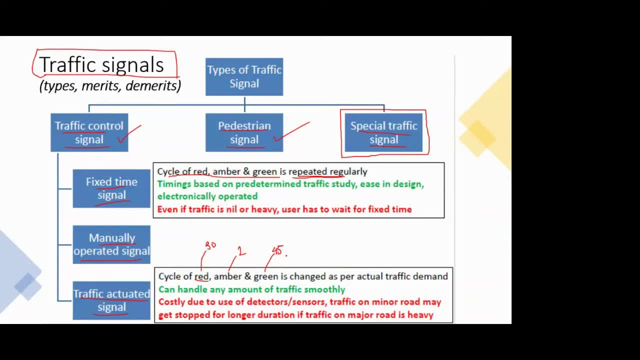 one way, sophisticated way, in which you can count the vehicle is you can have a videography survey and then you can feed that video to a software and that software will just segregate that what is the type of vehicle or how many vehicles are traveling on that road. so same way you can use 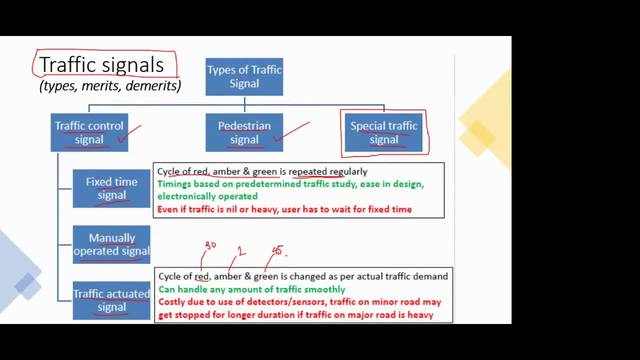 that over here and it is interconnected, that whatever is the live feed of the video, it is connected to the software. it analyzes immediately and then if it sees that there is no vehicle, so it will just give a green light to that road which is having, or where, a single vehicle or two, three, 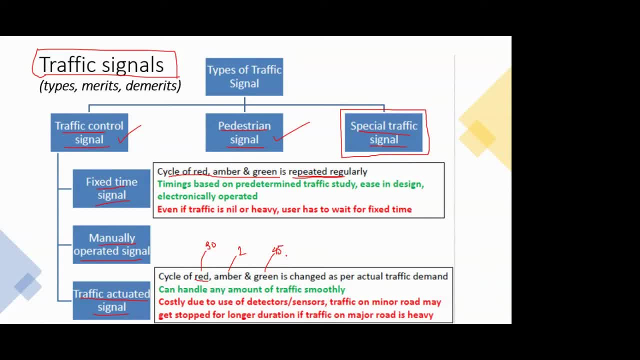 vehicles are approaching. okay, so that is a traffic activated signal and the same signal when it's a day time. so again, it will act accordingly that whichever road is having more congestion in it or more queue of vehicle is seen. so there the green time is increased and 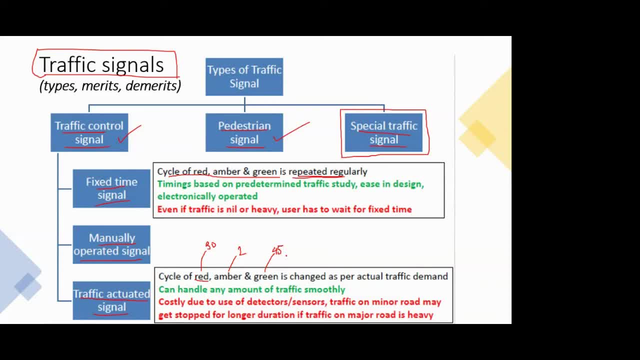 the another road, where it might be a minor road and the number of vehicles are also less, so there the red time is increased a bit. so in that way the traffic is controlled, and that is traffic actuated signals. so in this a lot of coding goes in, because you have to write an. 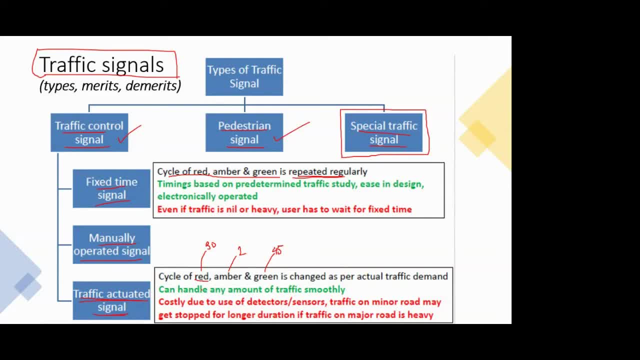 algorithm that if this happens, so what should be the decision taken? if that happens, what should be the decision taken? okay, so this is still picking some pace in india. it's not much seen everywhere. okay, wherever they have installed, they have installed. they had installed at a couple of locations in pune, also near napster, but that was on trial basis and 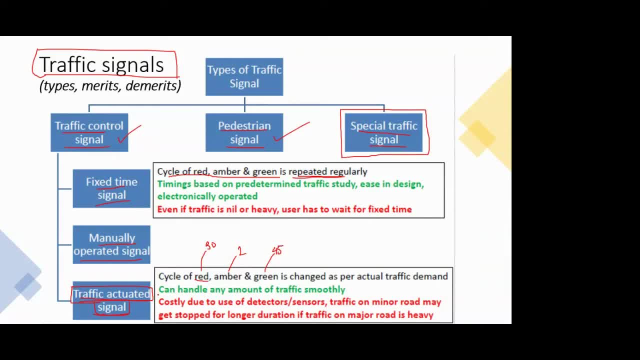 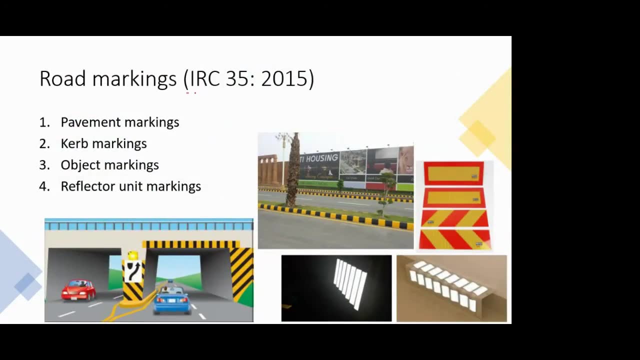 i don't know what happened to it, but now to it's the metro construction going on over there, so the signals are not working anyway. okay, so this is the discussion related to traffic signals. then comes the next control device, that is, the Mummer road markings. now, again, you have a special irc code for it, as you had for the traffic signs. 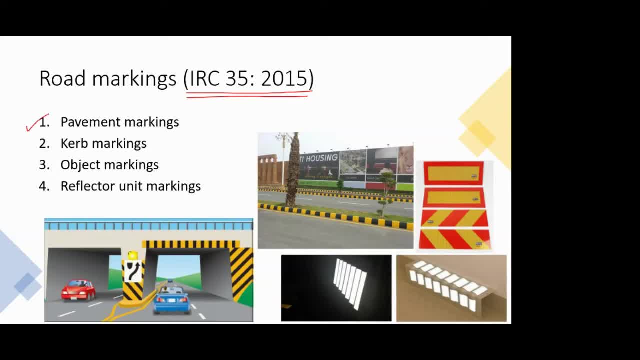 so in road markings you have four categories: the pavement markings, as in the ones which you can see on the pavement. so in this picture, whatever line i am highlighting, so those are the road markings. then you have curb markings. curb markings, as in whatever the median or footpath you 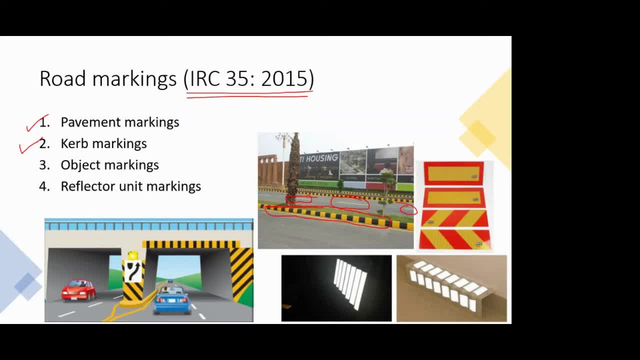 have so you can see, or you might have seen. it's colored in white and black or yellow and black. so that is the curve marking. so to demarcate that. okay, this is the curve. now, this might not seem important during day time, but at night time it is very important. 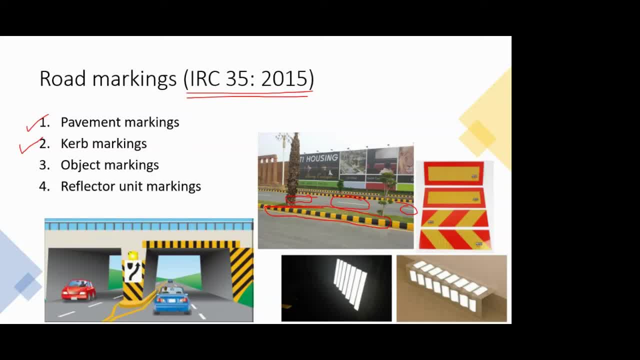 so that there is no mishap of any vehicle entering the footpath. then the third type of road marking, it is object marking. now, again, this you can see in the figure bottom left figure, this one which i am highlighting. so wherever you have an underpass, so there is a height restriction, so you can see such kind of 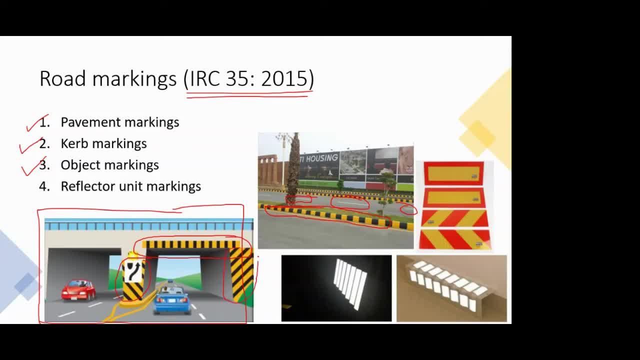 paints or painting done over there in yellow and black stripes. so those are the object markings. that's, there is some object and you have to warn the driver that, okay, you don't have to go into this object, you have to accordingly adjust your direction. so that is the object marking. and the last one is reflector unit marking from the name. 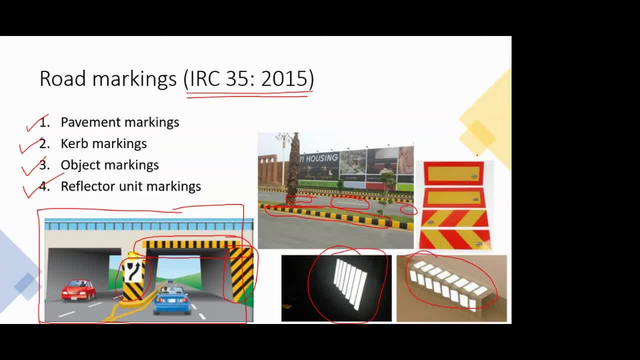 itself. you can guess that these are very much useful during the night time driving. so they will help you to demarcate some obstructions or some, some median suppose, or some curve. so they'll help you in that certain sense. okay, so let's move back to the next topic. and for Wyoming road markings. 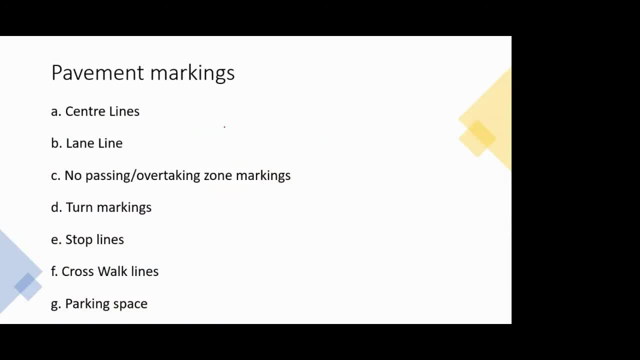 basically, these are the road markings. this is not a wither marking, it is a sighting marking. this is the Leslie brown and MATTE road marking. now this is bamboo mark, okay. or in this dotted line also, if the gap is more so, that also has some different meaning. 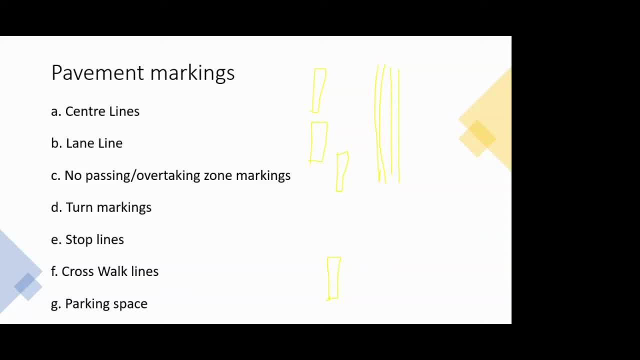 so now i'll not go into detail of all this because then again the irc code for the marking itself it is over 100 and 200 pages, so it will not be possible to tell everything. so you can just again go through yourself, do a self-study and get to know about the pavement. 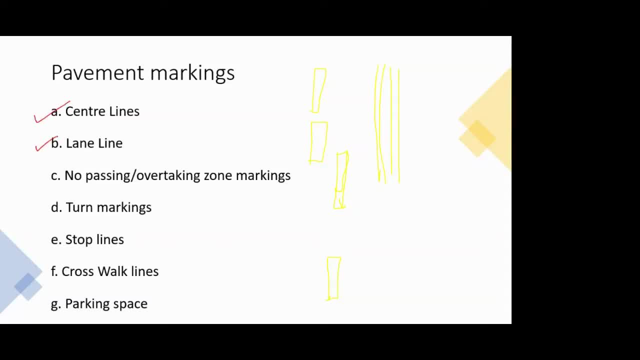 markings. so in that it is included center lines, lane markings. okay, then overtaking zone markings or no passing. so this is a no passing when you have a double solid line. so that means you are not allowed to overtake on that road. so even if there is a, there is not a sign of overtaking. 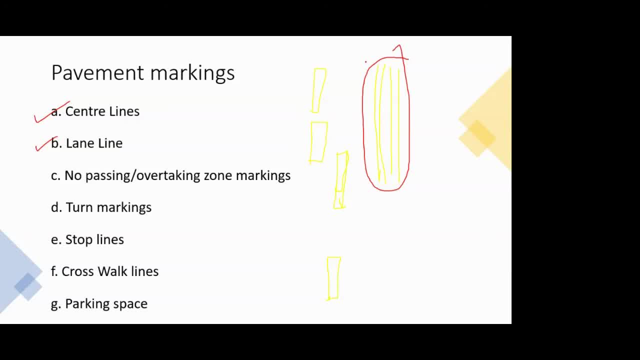 prohibited. but from the marking also you can come to know that. what is the way in which you have to drive on this road so very less at. i am very sure that almost 99 of the people don't know the meaning for the road markings. that why? 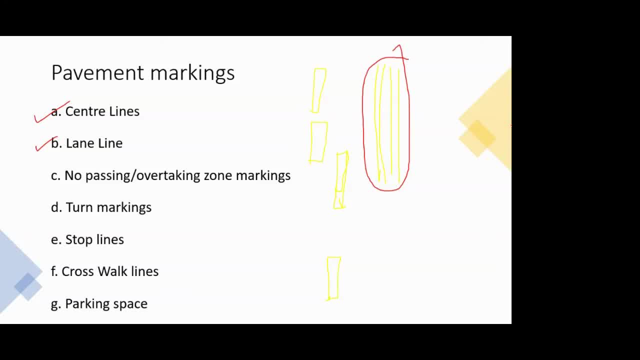 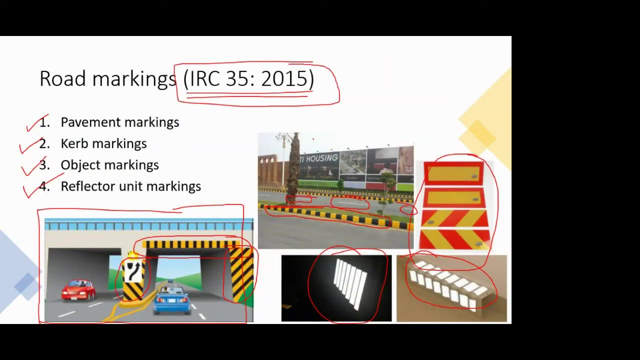 it is a continuous line. why a double continuous? and sometimes it is also like this key: you have one side continuous and one side, uh, dotted or dashed line, so this also has a different meaning. okay, so when you go through this irc code, you will come to know that which markings you have. 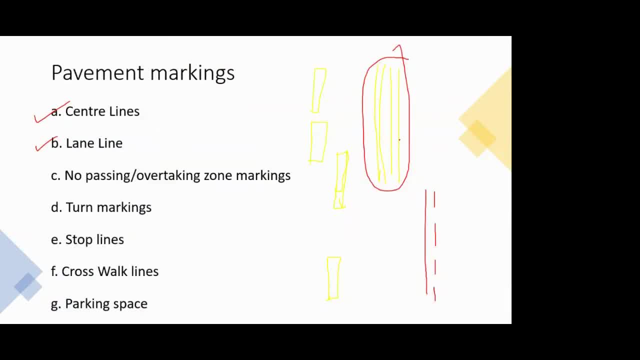 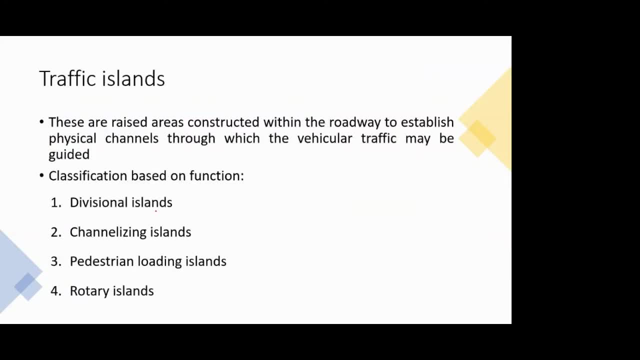 to follow in what way, and then that will make life easy for you whenever you travel on the road the next time. i am very sure about it. so just go through that irc code and the last traffic control device that you have is traffic islands. now, traffic islands, it is something that you have seen. 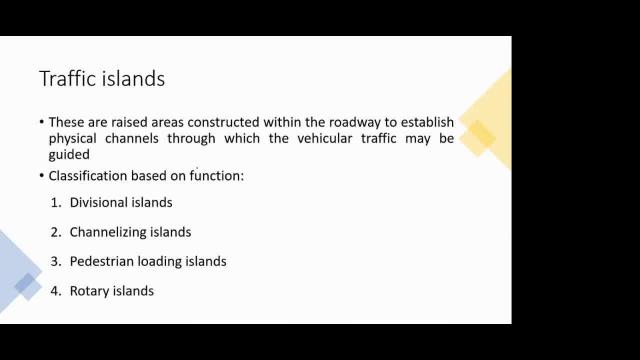 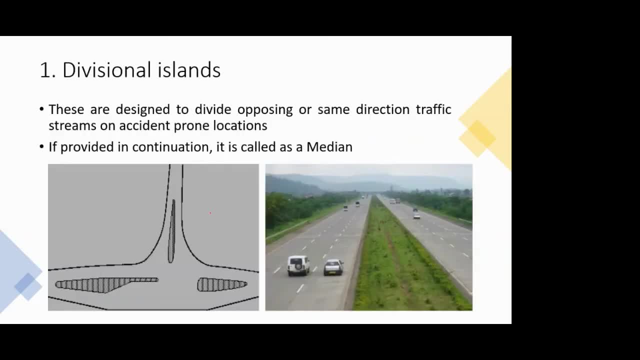 in your everyday life, while traveling, but you just don't know the technical term for it, that this is called as a traffic island. okay, so in that you have four categories. i'll go sideways. so first you have divisional island. now divisional islands. from the name itself, you'll come to know that it divides something. 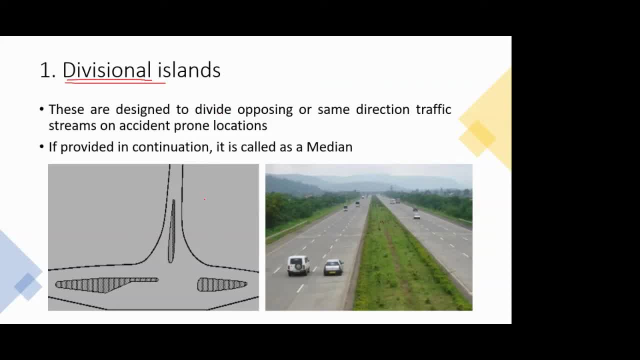 okay, and that's the exact purpose of that island. so on the left side, the photo number one, or figure number one, if you see. so it's a line drawing and whatever these markings you see which are shaded. so these are the divisional islands. now, what they do is they divide the flow of the traffic. 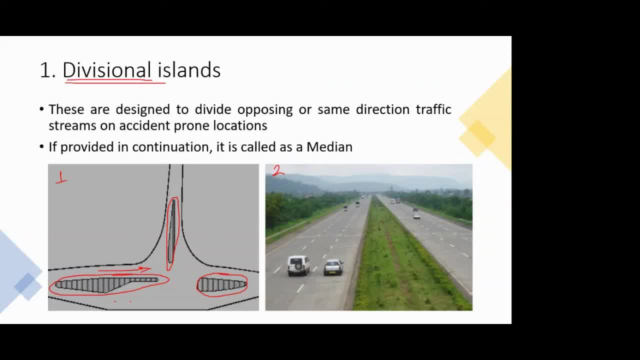 in two directions. so might be. this is for the up traffic and this is for the down traffic. so in between, whatever is the area they have developed now, it's not at the road level, it's a bit raised level. so that is nothing but divisional island. and if this divisional islands, 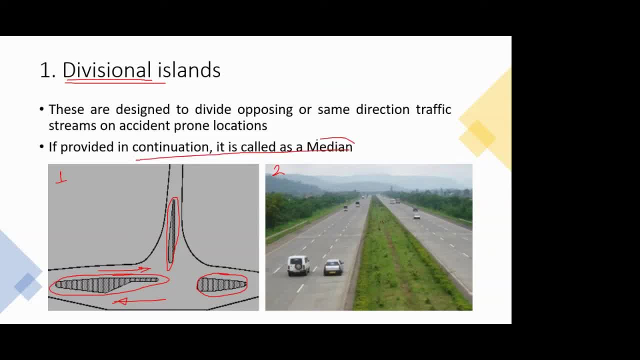 are continuous, then they are called as median, or what you all people know till now, uh, what we call a divider. so that divider is nothing but median, and this photograph on the right side you can see. so this is the median. okay, so that median is a type of divisional island. not always a median is continuous or not always. 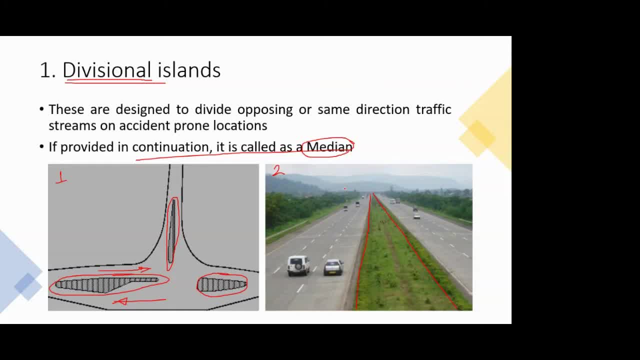 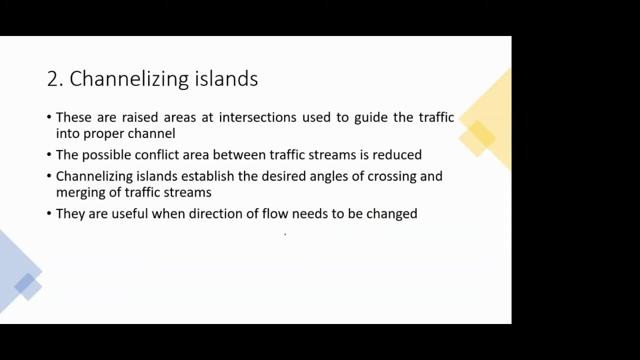 a divisional island is continuous. sometimes it's discontinuous as well, but that is also under the category of divisional islands. okay, and only when it is continuous. you call it a median, then the next is channelizing island. now these are some interesting features that you have on a road which help you control the device, control the flow of your traffic. 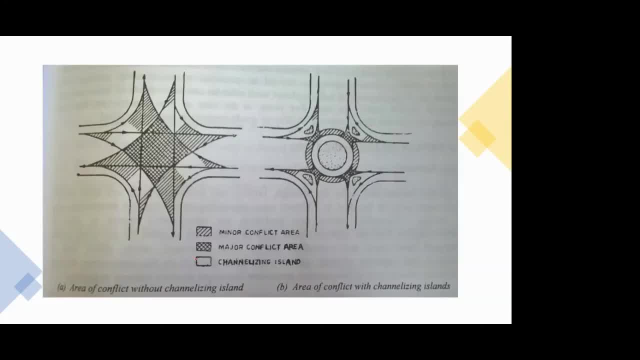 okay, so now, what are these? is suppose i have a. i'll give you an example. so in this figure, the left one, it is a four leg intersection without any channelizing island. so this was what i was saying, that if you have a two-way, two road, two-lane road, and if you mark all the directions, 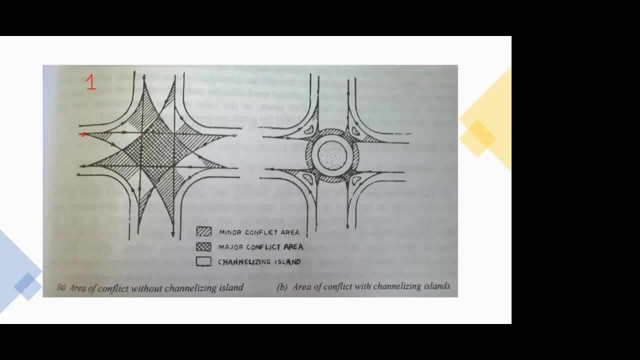 so you will get all this. you see, you can get all these conflict points over here. you can see this, this conflict point in this figure, very much clearly now, as I told you that, as a traffic engineer, it is a challenge for you to reduce all these conflict points. so how will you? 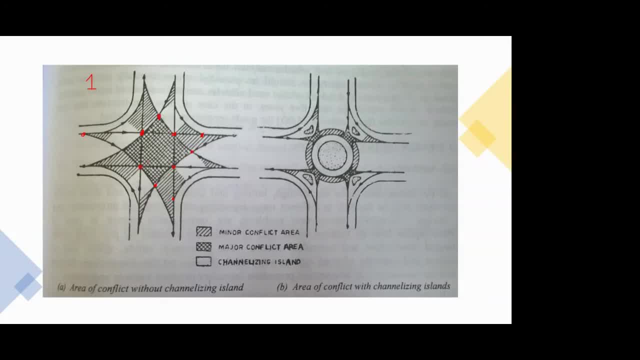 reduce it. so one of the best methods for reducing a conflict point is a channelizing island and what they have shown in this figure, if you say this legend. so the single directional hatching is for minor, minor conflict area and the double directional hatching is for 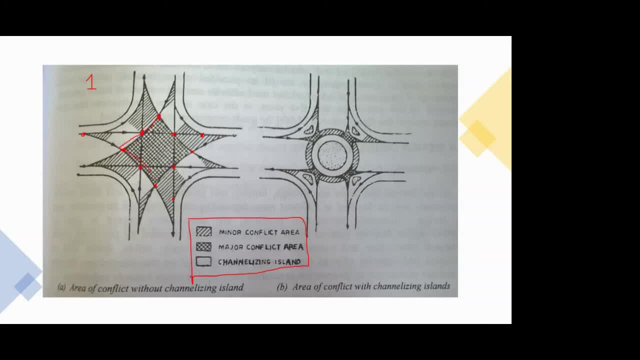 major conflict area, that is, the center portion of your intersection, where almost all the movements they cross each other. so now this type of intersection is always at a risk of going into a traffic accident, even if there is a traffic signal. we know that in India, how many people follow the traffic signal? 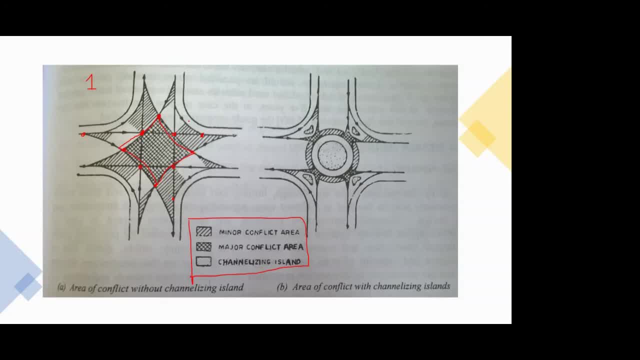 traffic signal very efficiently. so, even if there is a traffic signal, there is always chance of a accident at such location. so what is done is this intersection is channelized, what you can see on the right side. so what they have done is they have introduced a rotary. 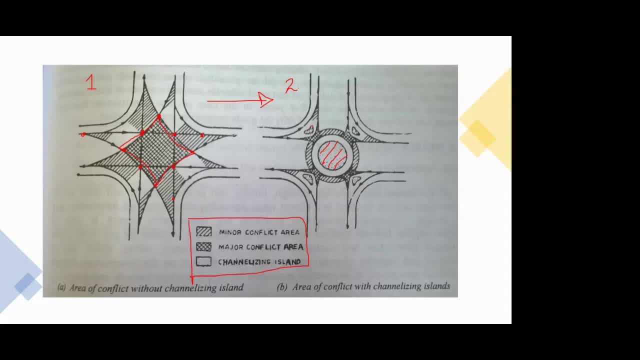 in between, or what is called a circle. then you can see this small islands. now what this small islands will do, They Will channelize your traffic flow, as in we have seen the diverging kind of traffic, or the merging kind of traffic, or diverging traffic, the ones who have to go straight. they will. 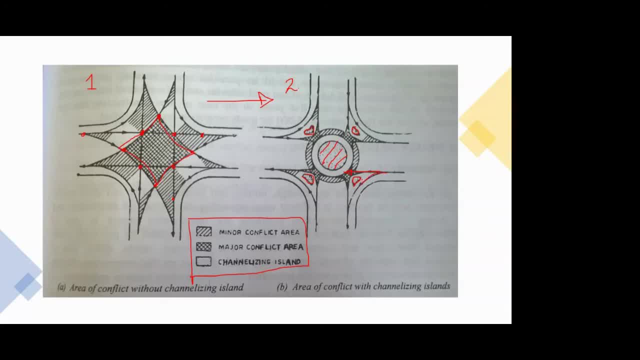 follow this path, but the ones who are supposed to take a left turn, so they will follow this part and bid in. between this, they will, or we will, construct a island over here. so this island is sort of an obstruction. so if you see your obstructions, obviously you will reduce. 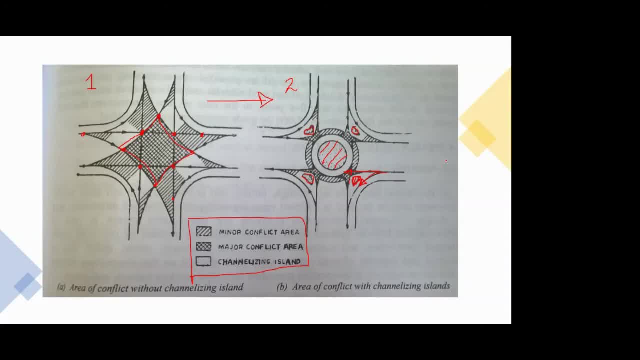 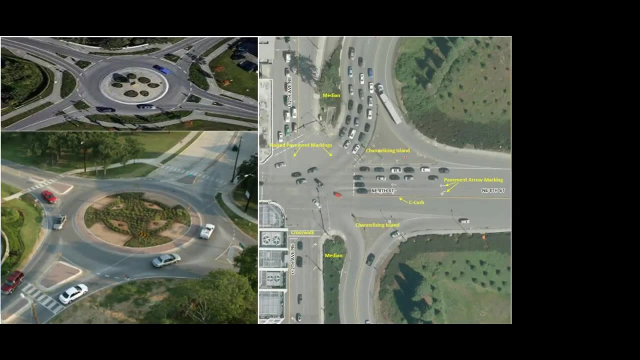 your speed and then you will take your turn. So these channelizing islands are a very effective way of controlling the flow and also the speed of your vehicles at the intersection. So in this slide I have shown you three photographs, and in each photograph you will see the channelizing. 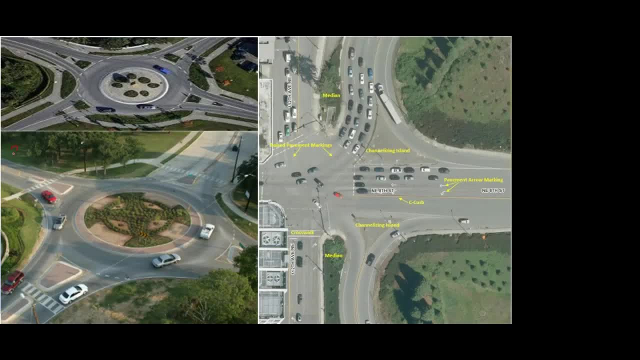 islands. So this is what I was talking about. let's see the photograph number two. so this is the rotary And this what you see here. these are the channelizing island. now, if you see, it is channelizing the flow such that there will be no intersection between these two, or even on the right side. 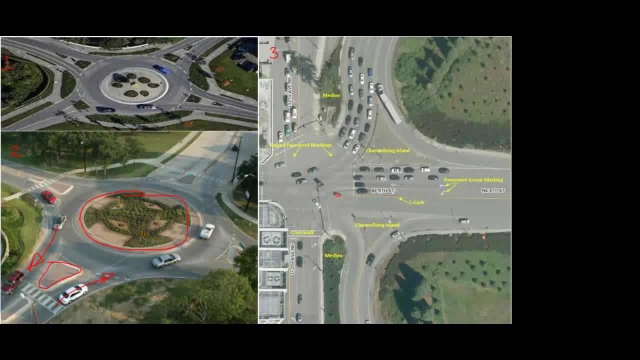 in photo number three, if you see. so just see this. this is the channelizing island. so now what it is doing is: Whatever is the flow which has to go straight, it will follow this side of channelizing island and the turning ones, they will follow this path. 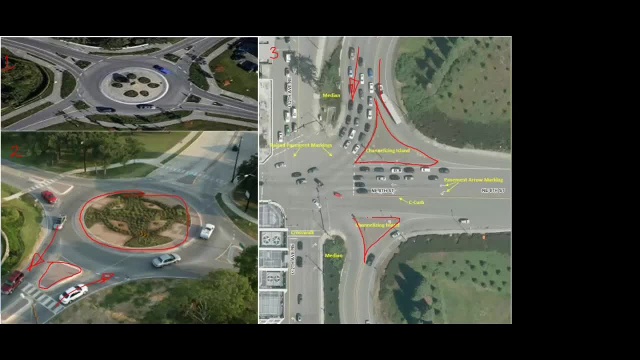 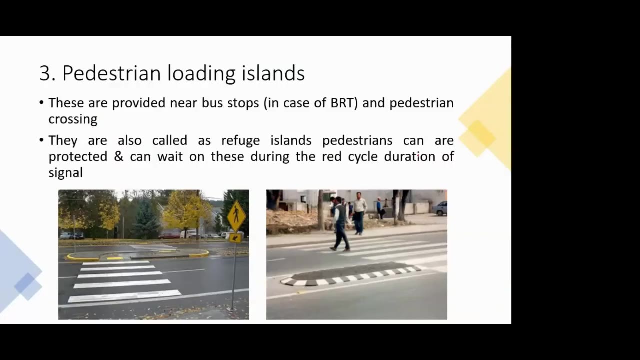 And same is the case here. you can see a channelizing island here itself, And these are the medians. now, these are the divisional islands that I discussed a few slides back. Okay, So this is example of a channelizing island. Then you have pedestrian loading island. 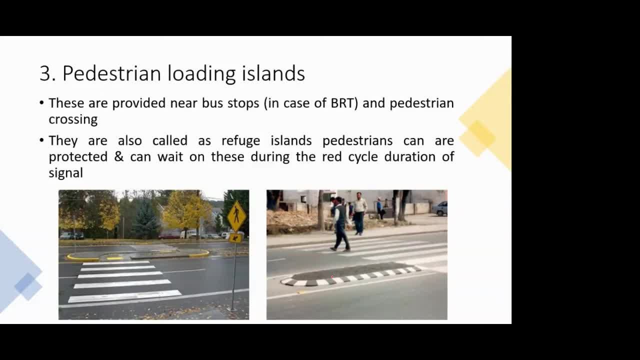 Now, these are for the purpose that whenever a pedestrian is crossing a road- So suppose the width of the road is quite large and then a pedestrian can't cross it in one stroke, or if you are at a student or you are at a young age- 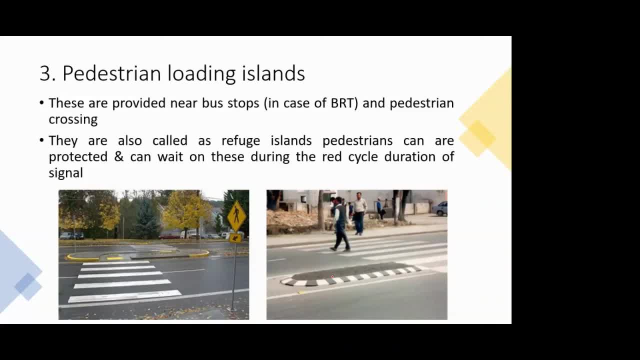 So maybe you can cross. but the pedestrians who have some walking condition, or they're having, Or their age is more so for them to walk for such a large distance in one stroke, and that means some speed. that is always difficult. So what is done is a sort of resting place is provided in the middle of the road, as in 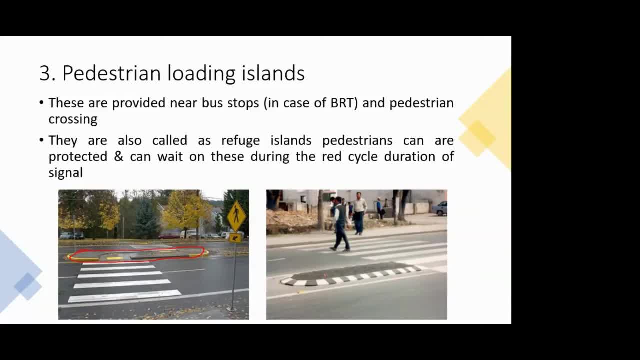 middle of the road, as in the median itself. So that is termed as a pedestrian loading island. So here you can see. so now this person is crossing the road, but if suppose there are vehicles, They are crossing here. So instead of standing over here, that person can stand at this location, and that will be. 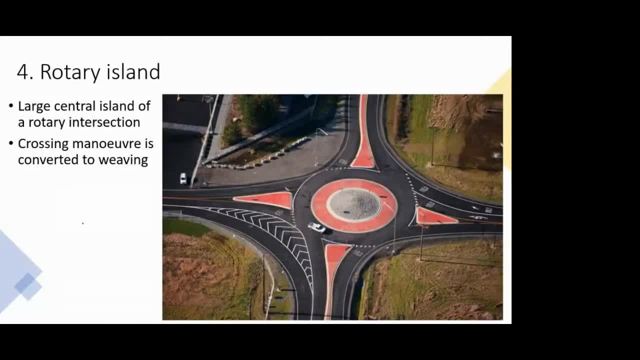 pedestrian loading island And they are asked: is rotary island? So again, rotary. now I have showed you before also. So rotary is nothing but when you have a large circle kind of thing in between and then you have channelizing islands at the same location. 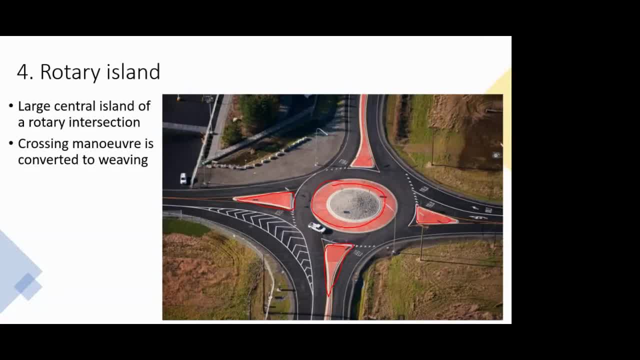 So that will be the rotary island Now. rotary island. the main purpose is now- whatever I had shown you at the starting, that you have crossing maneuver and you have a weaving maneuver. Weaving, as in the two movements they can go simultaneously. So that happens in a rotary. 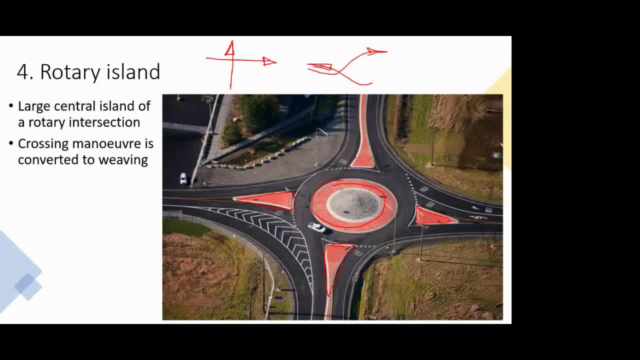 So now here, if you see. So this is a right-hand drive country from where this photograph was taken. So now, This vehicle- it is, maybe it is going to go in this direction, and there is another vehicle which is coming from this direction. So now what will happen is they need not stop. one of the vehicle need not stop. 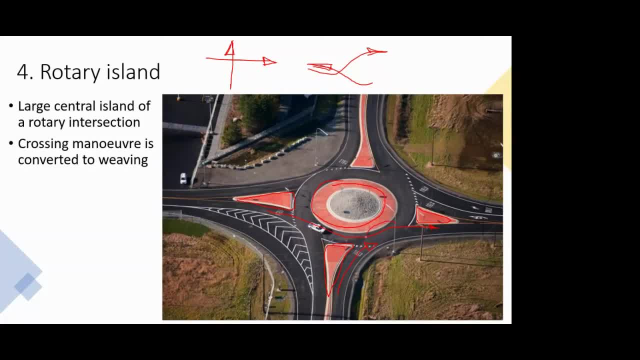 So both the vehicles can go simultaneously. But whatever is this common portion, viewing portion? So the curve is adjusted, this radius is adjusted in such a way that both the vehicles will reduce their speed and then one of the vehicle can easily pass and go to the desired direction. 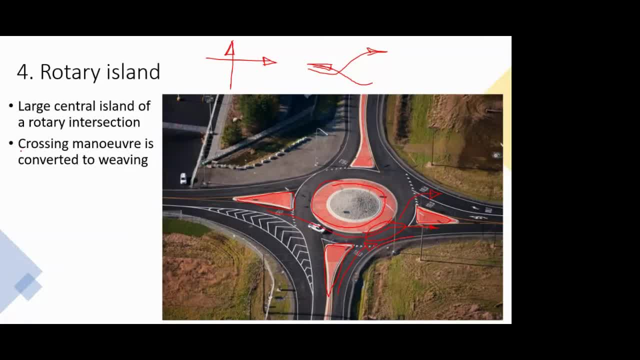 without the another vehicle stopping. So the main theme behind rotary is that crossing maneuver it is converted into weaving one. So we are not stopping anyone, but we are only slowing them down purposefully. So that is the main thing about a rotary island. So this, what you see in the center, that is a rotary island and this channelizing islands.